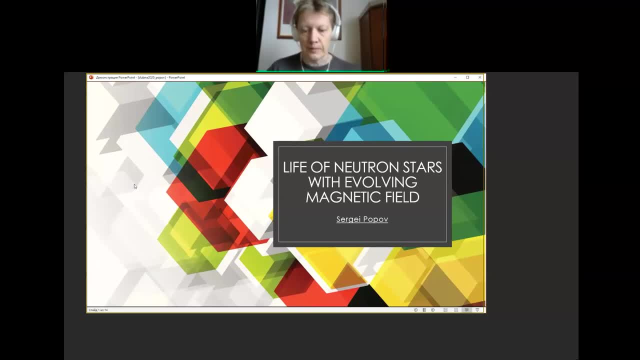 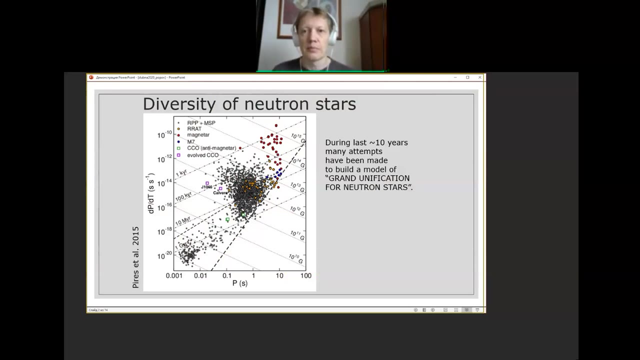 so, taking all together, I hope that this fits the general idea to present some interesting physics, also related to very interesting observations. So let me start. Let me start with some brief introduction of diversity of neutron stars. Neutron stars have been discovered more than half a century ago as radio pulsars And 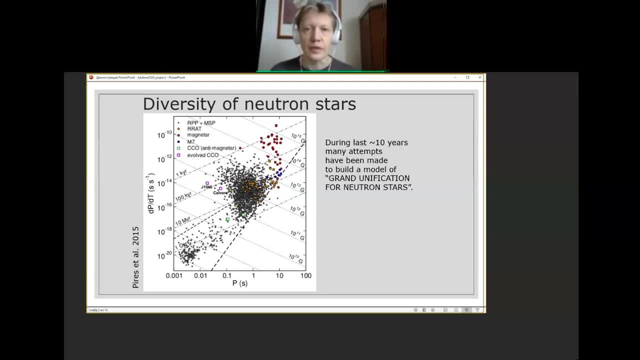 quite rapidly it was established, that it was accepted. I would say that neutron stars are born as radio pulsars, similar to their well known crack pulsars, And these are typical, even most typical, main representatives of all the horump neutron stars. 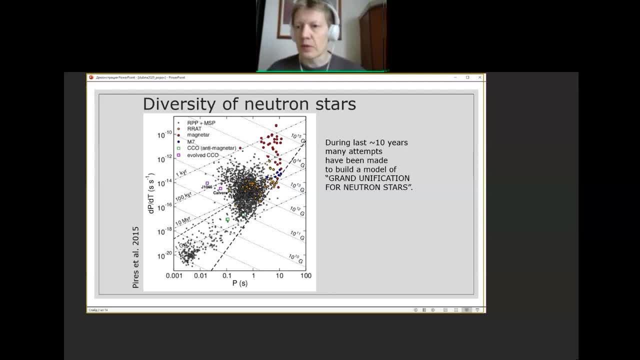 But starting from 90's, as you may be, not during the last ten years, but on a long period. Sorry for this misprint. Starting from the 90s, it became clear that young neutron stars can appear as sources of very different nature. Typically it is shown on such p-p-dot. 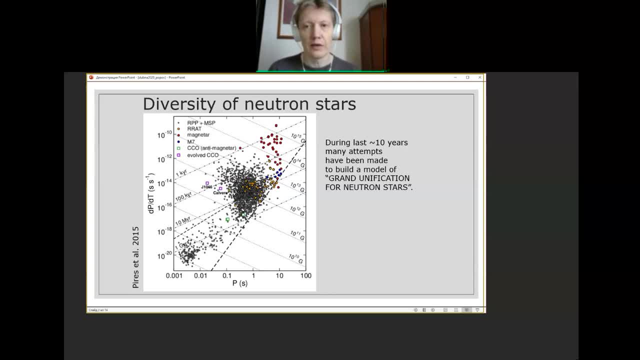 diagram. On the horizontal axis we have the spin period of neutron stars and on the vertical axis the first derivative of the spin period, so p-dot. This is a very useful diagram because on one hand it is 100% observational, so it's very model-independent. On the other hand, 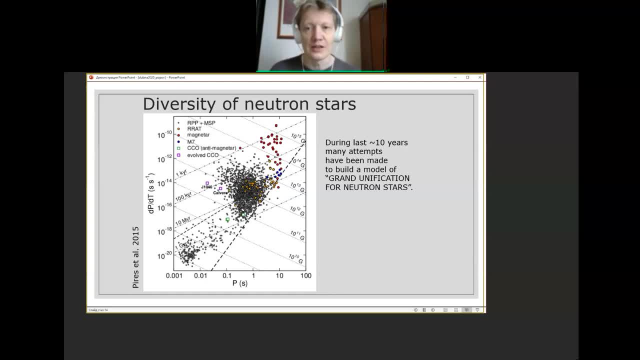 you can use models to draw additional lines on this diagram. I'll briefly explain what lines you can use. You see, in this plot There are many types of neutron stars. From the observational point of view, the most numerous neutron stars are radio pulsars and they are shown with black. 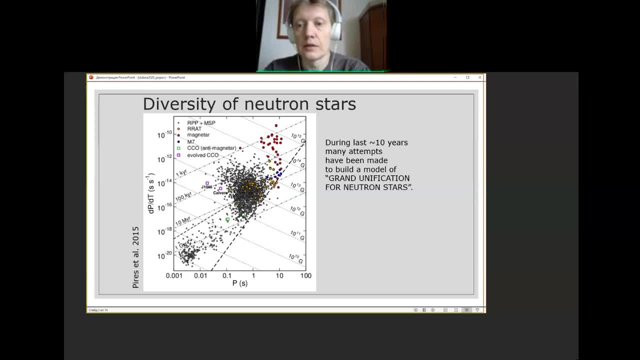 dots, The main crowd say, of these radio pulsars have typical periods about a fraction of a second- They are close to one second- and period derivatives about 10 to minus 15.. This makes radio pulsars very stable plot, and especially if we look at the millisecond pulsars which will not 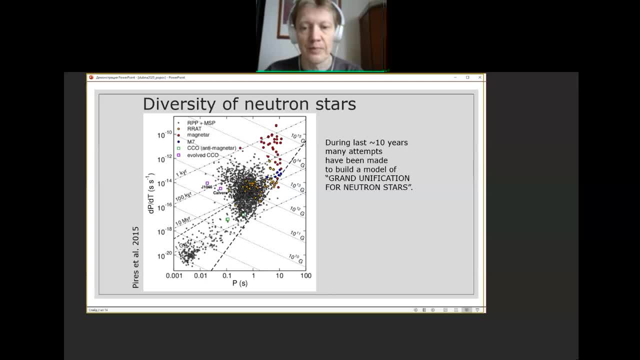 be the subject of my presentation. They are in the bottom left corner. They are really very stable rotators and quite often it's disgusting that they can be potentially used as a spin. This is the standard, the basis for the standard of time. 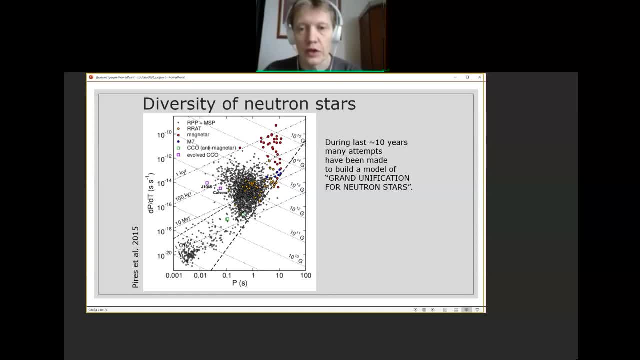 But in addition to these radio pulsars, which again are numerous, we know many other types of neutron stars. so let me start with magnetars. They are shown in the top right corner of the diagram shown with red circles. Magnetars are known for their high magnetic fields. and also attention to the final structure of the halo In a huge case. I'm sure you will not remember the name of any magnet, but magnetars are fictitious. Your magnet is like a star. You need a magnet or an atom or something else. 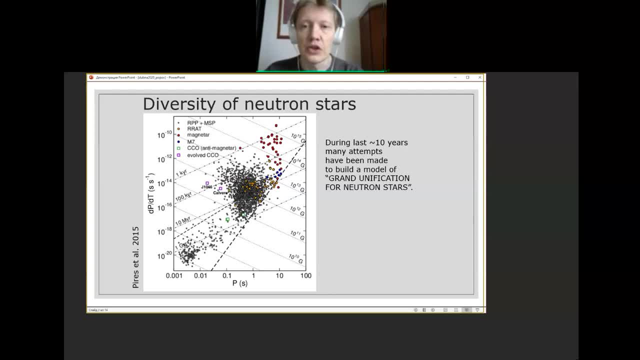 and this would be part of the presentation- also for their spectacular observational appearance for many interesting phenomena related directly to the energy of their magnetic field. Then there are other types with orange dots, rotating radio transients shown with blue dots, so-called Magnificent Seven. 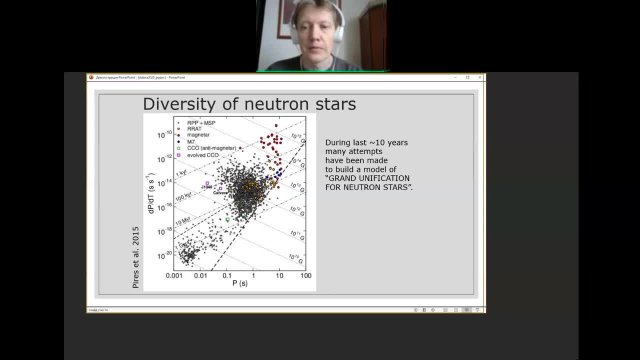 seven nearby cooling neutron stars. These are quite interesting sources because they really look like predicted, say, neutron stars. Neutron stars have been predicted in mid-30s by Bade and Zwicky and they were predicted as 10-kilometers-sized objects, born hot. 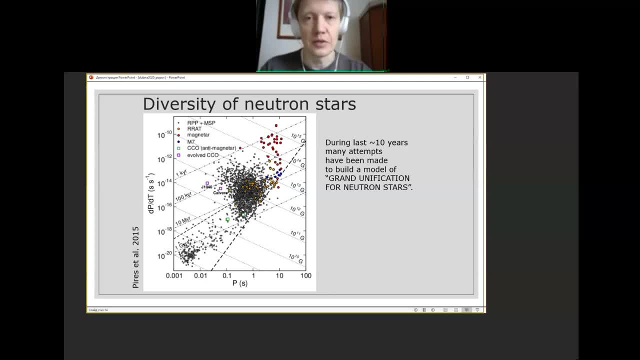 So they mean predicted observational appearance, and so neutron stars was the thermal emission and Magnificent Seven sources of this time. Then there are some other examples and of other types of objects. We'll come to them later, And since it was realized that there are many different types, 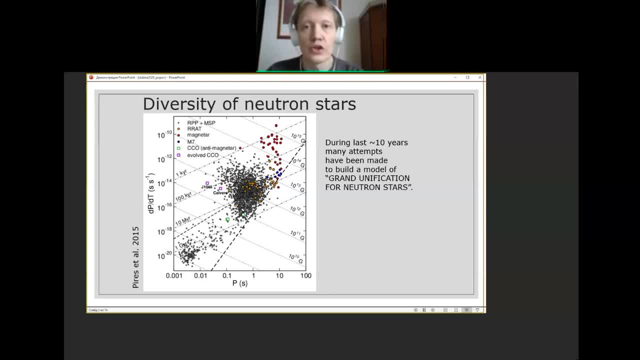 of neutron stars. then the natural question appeared why they are so different. So, really 10 years ago. that's why that number here. 10 years ago, in 2010,, people started to talk about grant unification for neutron stars. 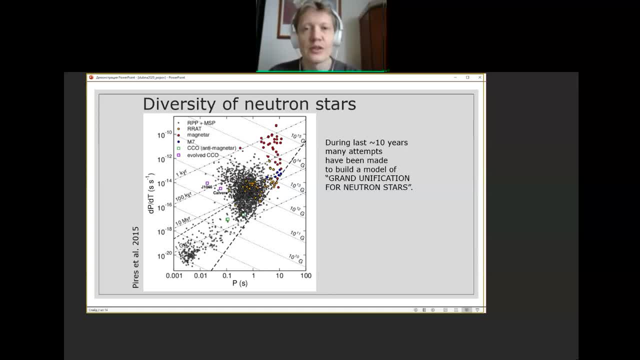 So the idea is to explain different types of neutron stars in one evolutionary framework, starting with some general initial distributions of different parameters, And this is an interesting and non-trivial topic, but it's a very interesting topic. It's a very trivial task. 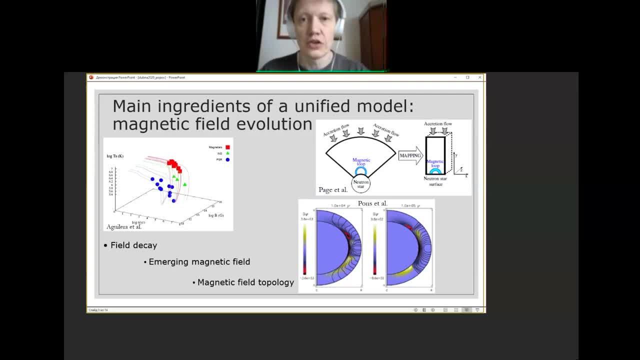 And now it seems that the main ingredient of such unified models is the magnetic field evolution. well, magnetic field properties in general, And there are several important points. I'll underline three of them. So the first, the main maybe point, is that the magnetic field is decaying. 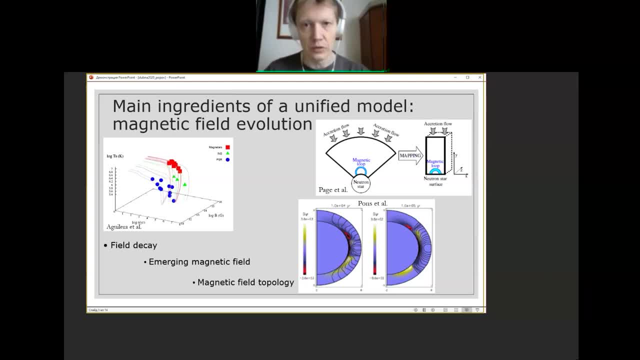 So magnetic field is formed, enhanced inside neutron stars, So magnetic field is decaying. So magnetic field is formed, enhanced inside neutron stars, So magnetic field is formed, enhanced inside neutron stars, But then generally during the lifetime of these complex objects. 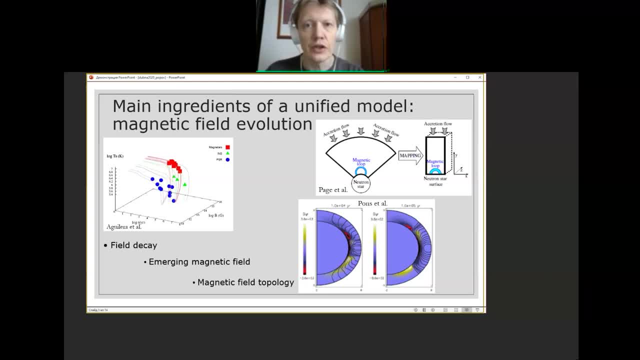 the magnetic field decays And the energy of magnetic field or the energy of electric currents, whatever you like, is released. It can be released gradually, relatively slowly It goes into heating or the crust of the neutron star, or it can be released in bursts. 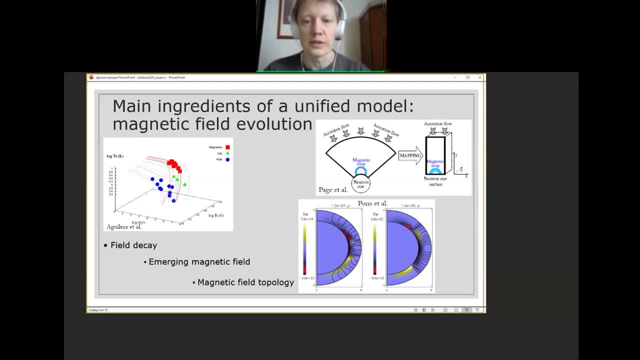 Then we can see really spectacular transcendental and magnetic field of a neutron star can be hidden. So inside the neutron star you have strong magnetic field. Everything is fine. But a relatively thin envelope can screen the magnetic field. So for the external observer, 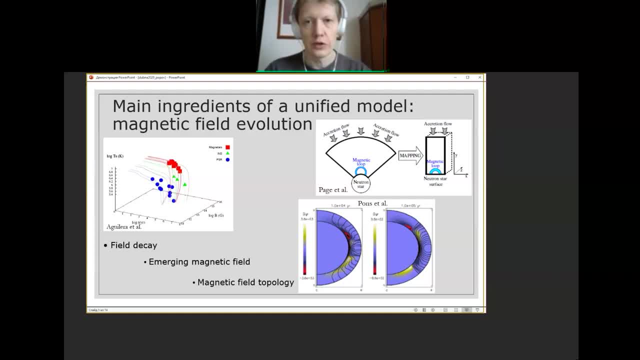 the magnetic field of a neutron star is not large And the magnetic field slowly can diffuse out And for the external observer again it looks like enhancement, like increase of the magnetic field. So this is this phenomenon of emerging magnetic field. Finally, it's very important to take into account: 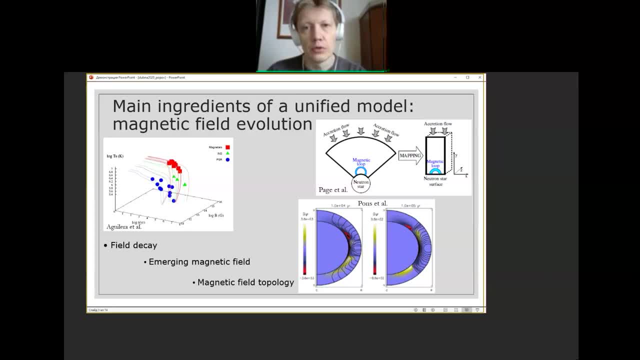 detailed topology of the magnetic field inside the neutron star, either in the crust, as it is shown in the picture on the slide, or also in the core, And I'll say a few words also about this. This is quite a recent topic. 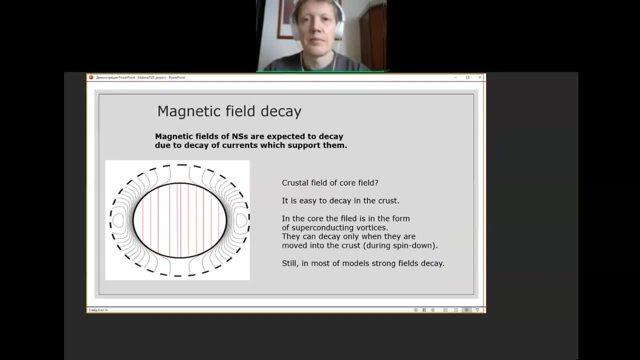 So magnetic field decay- Mainly I'll speak about this particular subject, but also two others will be also mentioned. So magnetic field decay. The structure of a neutron star can be at first described with two main regions: the core and the crust. 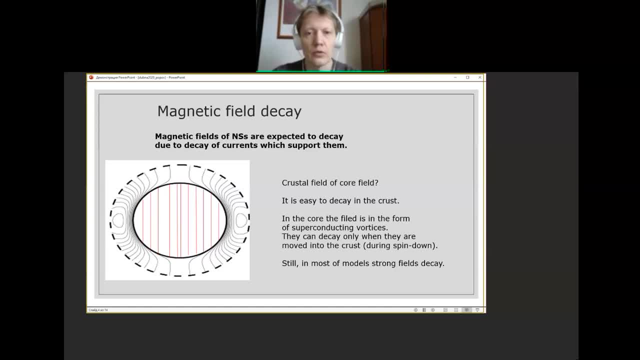 And the physical conditions are very different in the core and in the crust. Magnetic field can be and might be present in the core and in the crust together. Still, physics in the crust is easier, is simpler And many modern models of the magnetic field evolution. 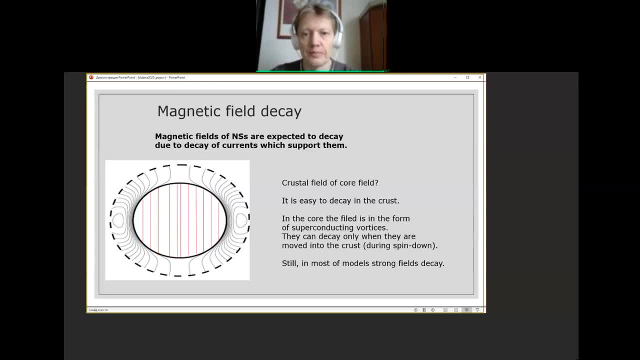 deals just with the crustal magnetic field. In the crust we have more or less normal matter. so there are electric currents. They support the magnetic field. In the core the situation is different. Protons are in superconducting state. 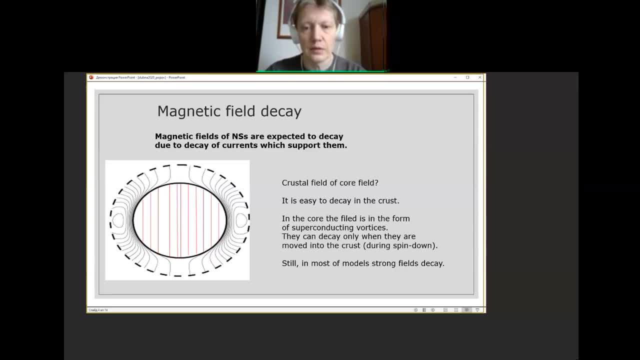 So the magnetic field forms quantum tubes, magnetic flux tubes, And this is quite a different picture And for quite a long time people pretended not to discuss evolution of magnetic field in the core. All people just use very simple, relatively simple models. 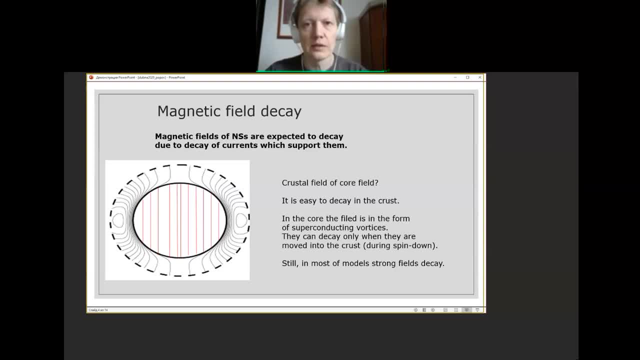 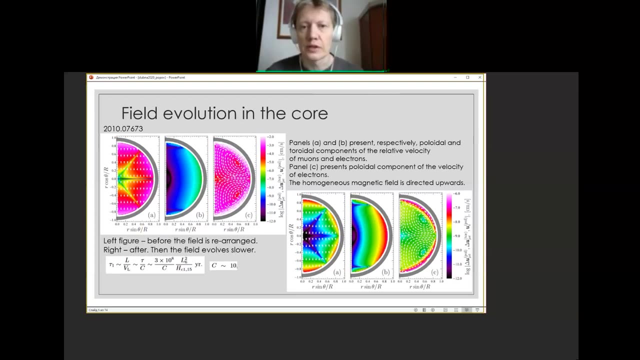 And in astrophysical applications they were not very often used, So people mainly focused on the crustal field evolution, And so I'll do it during my talk too. However recently- this is really recently- I noticed the number of the paper in the archive. 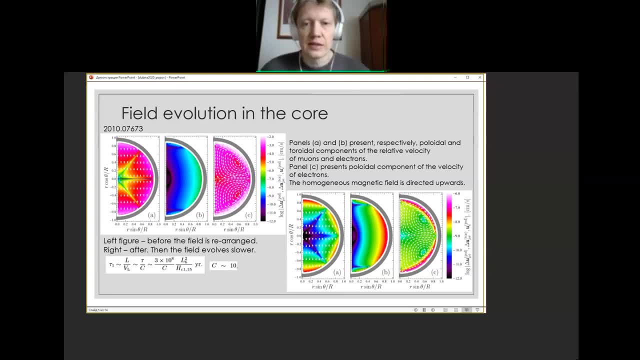 So it's October this year. It appeared less than a month ago, So very recently. people started to attack the problem of the field evolution in the core on a new level. This is done by a group in Yoffe Institute in St Petersburg. 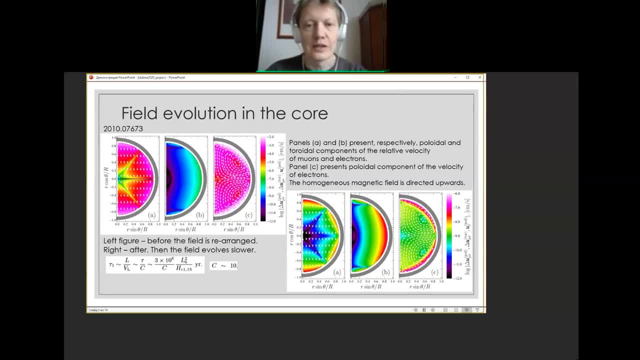 And this is really a beautiful piece of physics. So if you are interested- I mean not in neutron stars, but just in beautiful physical problems- I strongly recommend you to look at this paper. I just grabbed two beautiful pictures. Actually, they represent 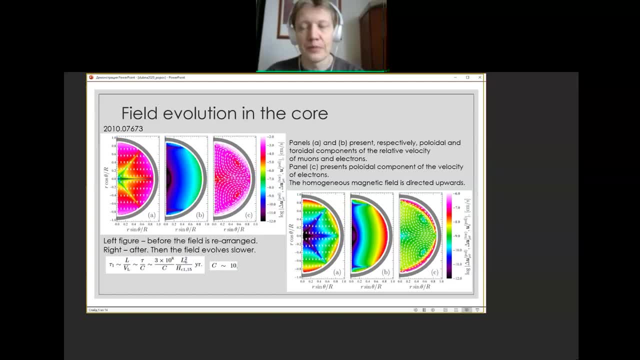 not the magnetic field structure but the velocity field of particles inside the neutron star. So plots are made for electrons and for relative velocity of muons and electrons inside the neutron star, And of course movements of these charged particles influence the magnetic field in the core. 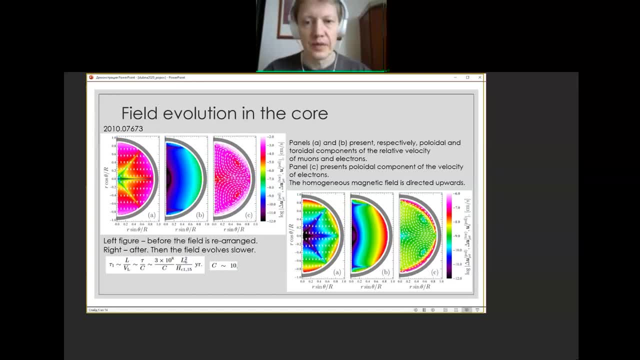 And, what is more important, they start to calculate realistic models which can find, and definitely will find, statistical applications, And they obtain important time scales And, yeah, let me start to introduce these time scales now. So, in the model of core field evolution, there are several periods: a very rapid initial period which depends mainly on the cooling of neutron star, and then another episode starts which is probably more important for astrophysical applications, And then the scale of magnetic field evolution is about. well, it depends on parameters. 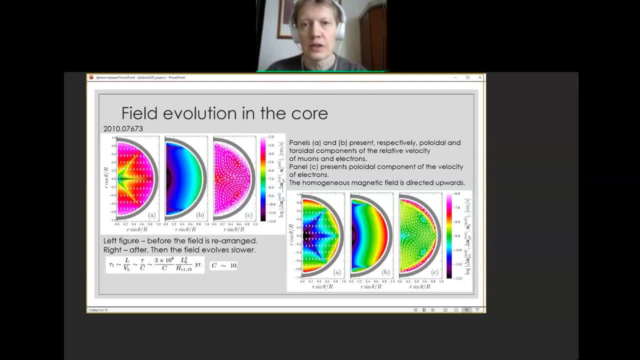 so it can be from several hundred thousand years at early stages up to tens of million years at later stages. This is compatible with typical ages of radio pulsars, say lifetime of radio pulsars, And it looks like we are standing very close to a new, maybe breakthrough. 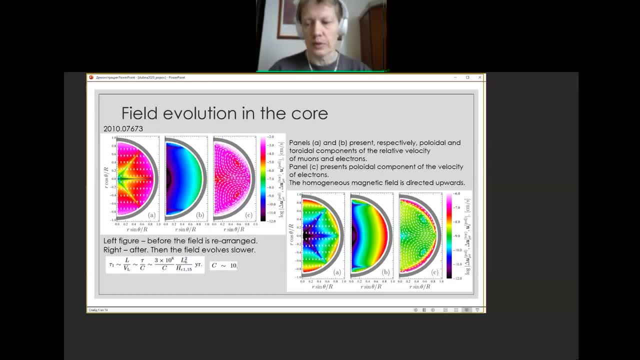 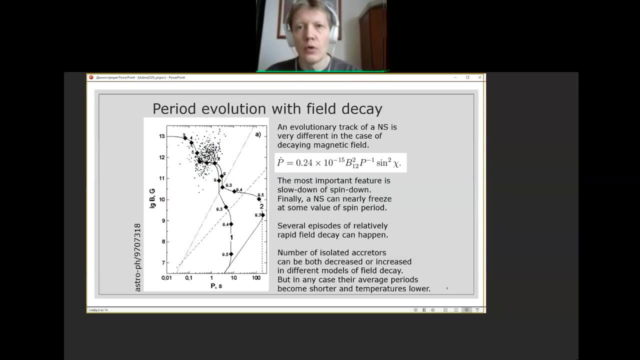 in studying evolution of neutron star's magnetic field. But mainly in the rest of my talk I'll discuss models of the crustal field evolution mode and field in the core, Independently on the position of the magnetic field we are discussing From the observational point of view. 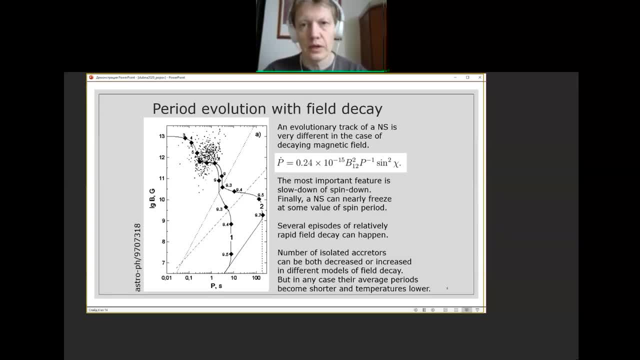 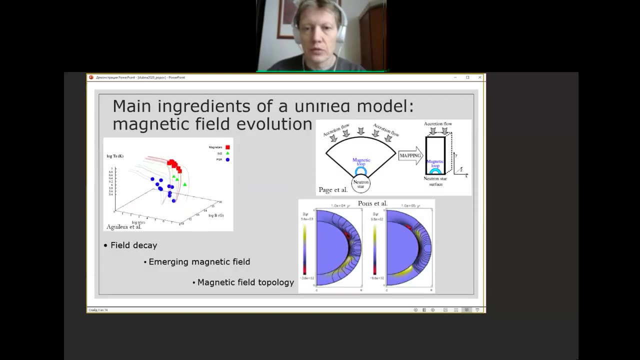 the first thing you observe if the magnetic field is evolving is evolution on the PP dot diagram. So this is more or less an analogous of the PP dot diagram. Let me maybe come back to the first diagram I showed to you. So here really, 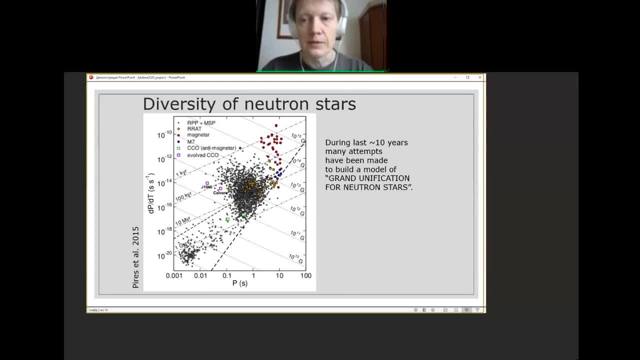 we have PP dot, but I promised to explain a few lines. So in the simplest model of neutron star, evolution, magnetic field is constant and the spin down of the neutron star is described with a simplified magneto-dipole formula. And then the life track of a neutron star. 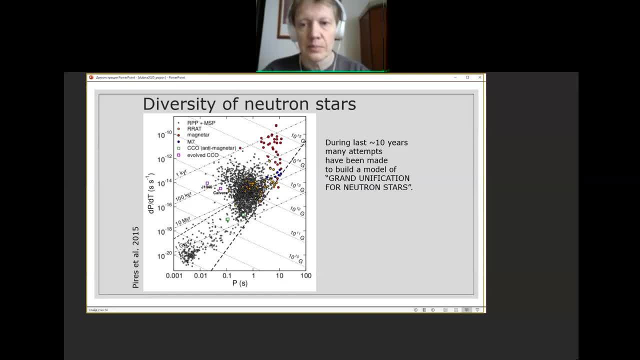 at this stage is a straight line in this plot And these dotted lines with marked values of magnetic field correspond to such evolution. So, for example, there is an evolution with constant magnetic field 10 to 13 Gauss or 10 to 12 Gauss. 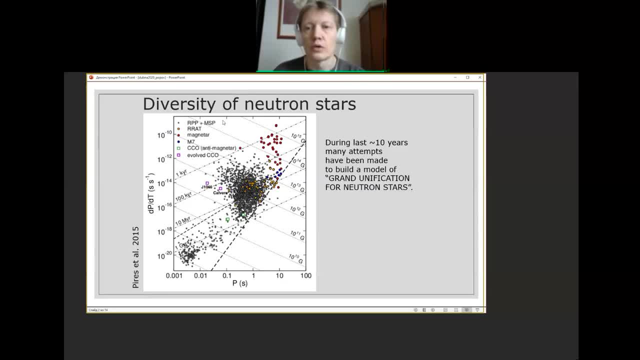 which is more typical for normal radio pulsants, or 10 to 14 Gauss passing through the magneto region. However, if the field is evolving, the situation is different. Here notice that you can, in the simplified model you can map one-to-one. 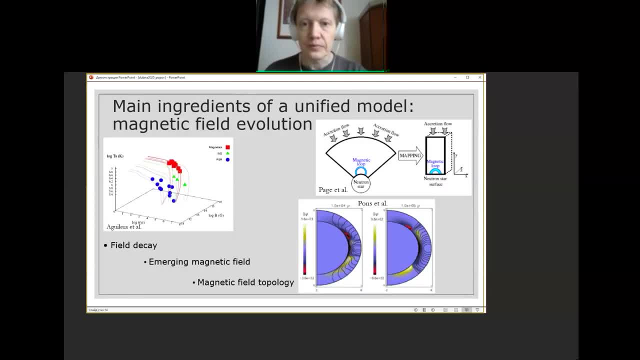 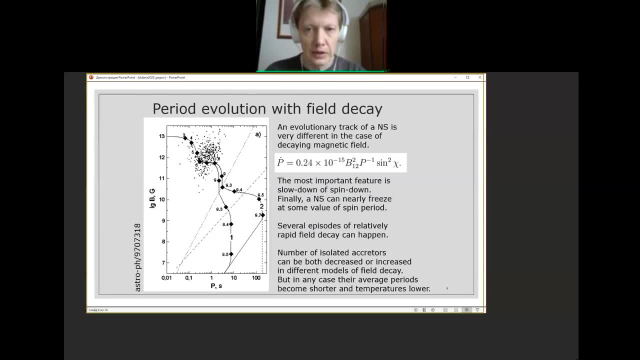 P dot to magnetic field So you can redraw this plot with magnetic field on the vertical axis. This is a dipole, external magnetic field of a neutron star, And so if the magnetic field is decaying then the neutron star is rapidly moving down. 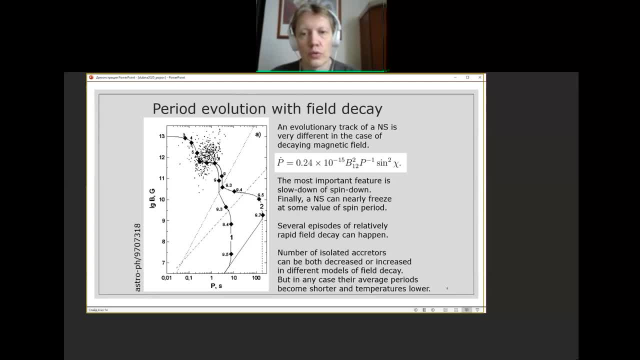 So normal evolution drives it to the right. If the field is constant then of course a neutron star just goes to the right. But with the field decay it starts to go down. The same would be in the P-P dot diagram. 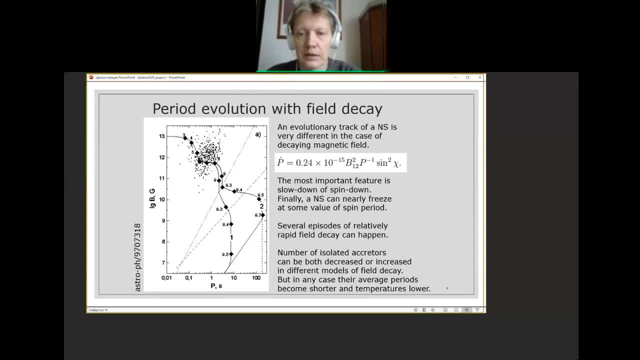 Also it starts to go down on the diagram, And here already it's taken from not very new paper. You can distinguish several episodes of magnetic field decay And this is quite important because indeed evolution of currents inside the crust of a neutron star. 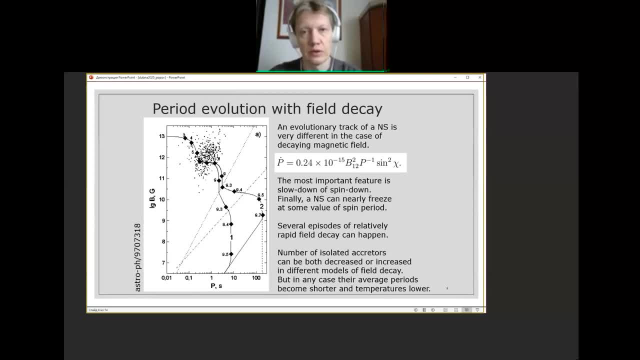 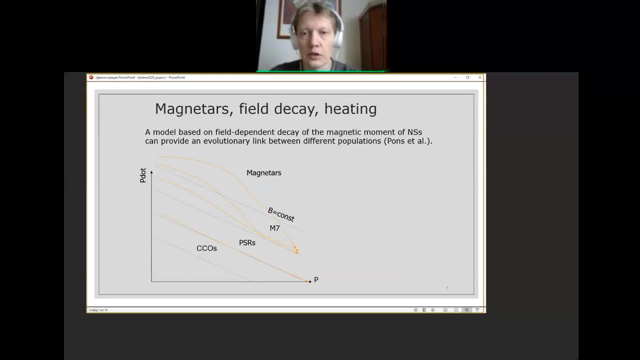 can go through several different episodes, So different physics drives magnetic field evolution at different stages. Also, magnetic field evolution in a neutron star depends on the magnetic field itself. It was not, I would say, so obvious from the first principles, but observations definitely. 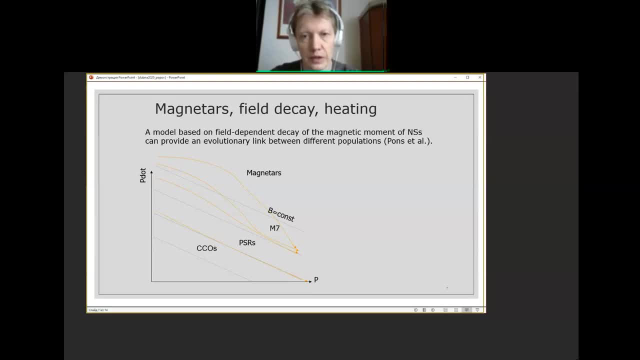 point towards this situation. Large magnetic fields evolve, decay much more rapidly And presently we definitely see clear signs of evolution, of magnetic field decay in magnetars, for example, And we, well roughly, do not see very clear evidence, and definitely we don't see clear evidence. 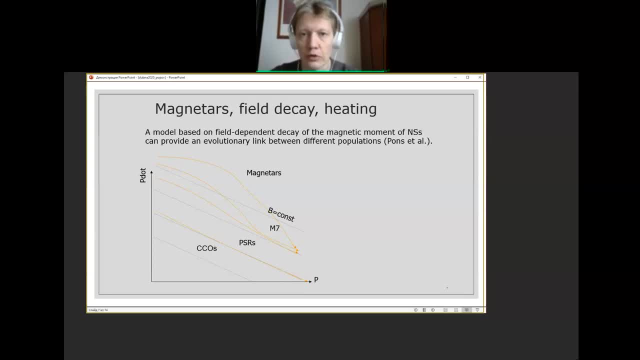 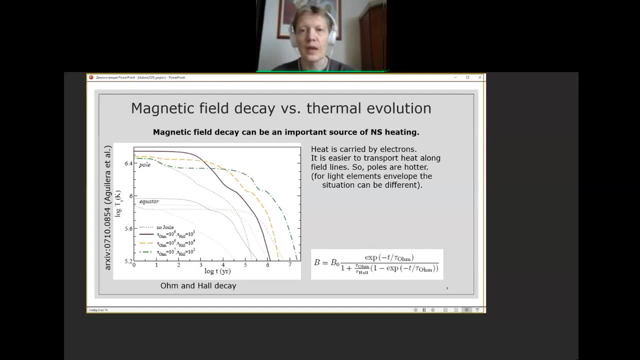 for long-term magnetic field evolution in normal radio pulsars or in other types of objects with lower magnetic field. What do we see in magnetars, for example? In magnetars, as I said, we have two main effects of the magnetic field: decay. 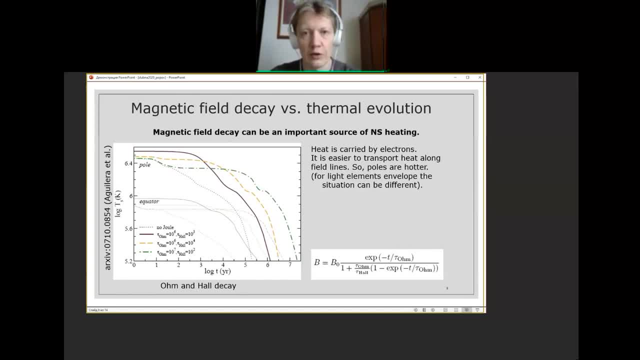 The first one which actually allowed to discover magnetars. magnetars in this sense were discovered at the very end of the 70s, mainly thanks to space observations by a group again from the Iofi Institute, another group, The group by 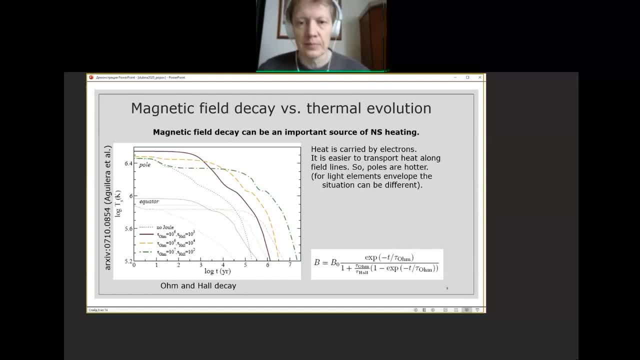 leaded by Evgeny Mazets at that time. So they discovered repeating bursts of several gamma sources and they discovered pulsations in these bursts. Pulsations are related to spin periods of neutron stars. So, step by step, it was established that these sources 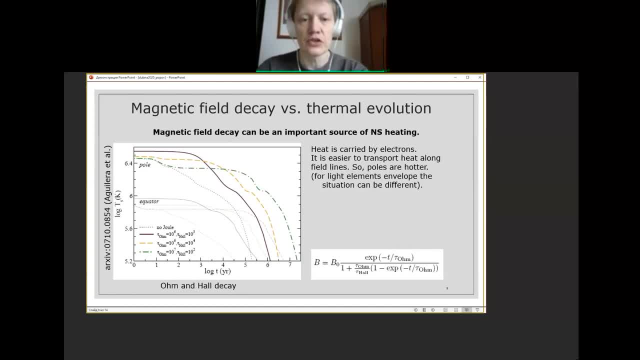 are strongly magnetized neutron stars and magnetic energy is released during these spectacular events. This is really spectacular. For a fraction of a second 10-kilometer neutron star becomes much- not just, but much- brighter than the whole galaxy. This is really splendid. 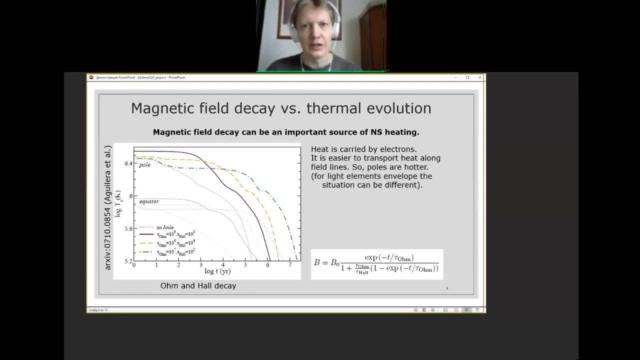 And in addition to this, in addition to this, trends were very strong. I cannot say catastrophic because they repeat, but still very energetic, explosive phenomena. There is a gradual magnetic field decay which just hits the crust of a neutron star. Then the heat is transported. 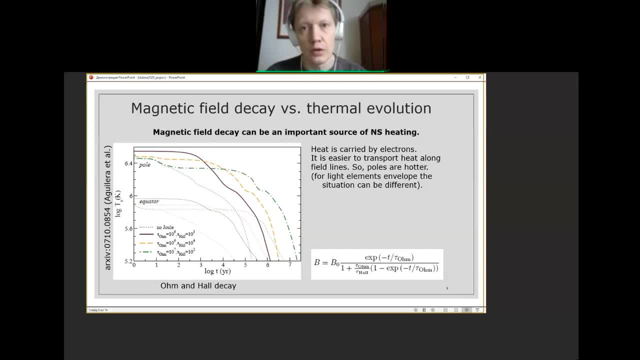 mainly, it is transported downwards to the interiors of neutron star and then it is lost due to neutrinos. This is actually a problem because neutrinos are very efficient in taking energy from neutron stars. Neutron stars are transparent from these particles And because of high density. 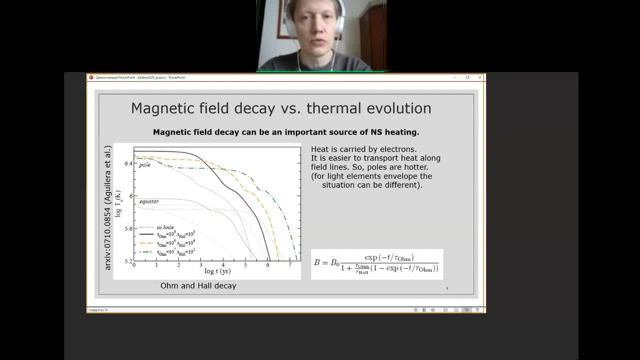 neutrinos are effectively emitted inside neutron stars. So neutron stars cool in a very funny way, not from outer parts, not from the surface, as it normally happens with everything with potatoes, But they cool down from their interiors due to neutrino. 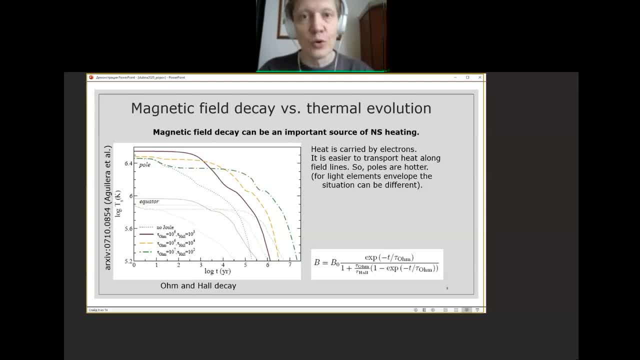 So neutrinos are the main cooling agents of neutron stars. Still, some heat is transported to the surface, transported by electrons mainly, And then we can observe these sources as thermal sources, And this is shown on this plot. So these are cooling curves. 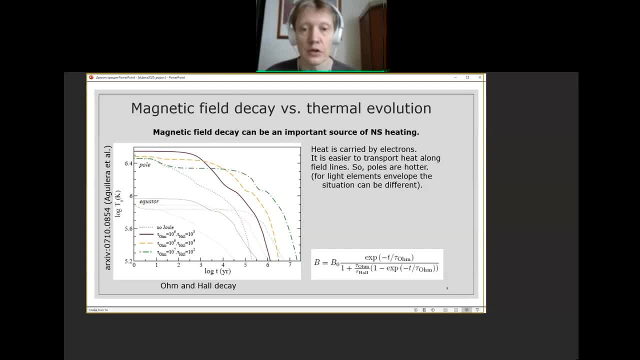 And what is shown is the temperature of different parts of neutron stars that they create around the decoll. This is, I would say, simplified model. It is just a model. Every physical model is simplified, in a sense, by definition in comparison to nature. 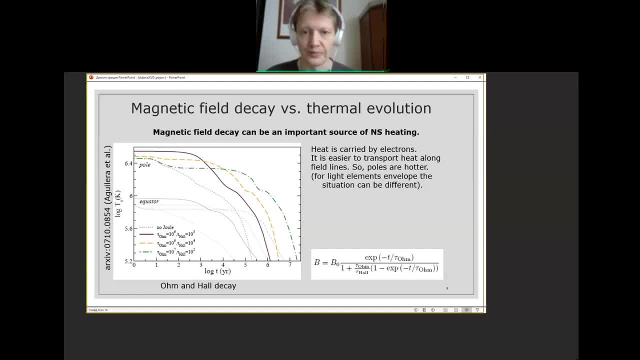 Still I want to underline that not in every model magnetic poles are hotter than equators. It is possible to make such a model where the situation would be opposite. Still we see that if there is a rapid magnetic field decay, then on the surface 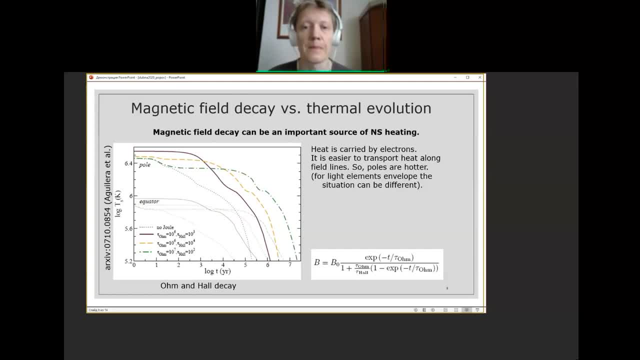 so on the visible surface of a neutron star there can be regions with significantly enhanced temperature. Temperature goes to the luminosity in power four. So even a moderate increase in temperature, say by a factor of three, gives you nearly two orders of magnitude. 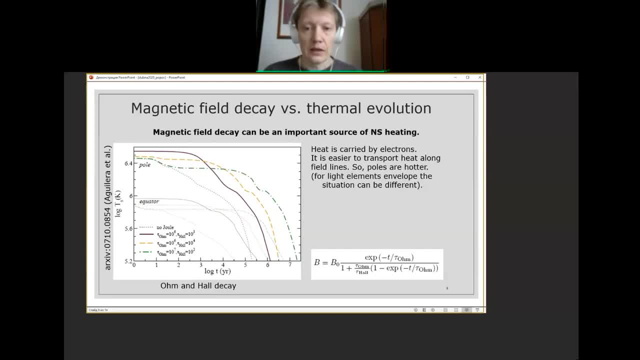 increase in the luminosity And for high magnetic field. this is calculated for high magnetic field. the effect is really strong And we observe thermal emission of magnetars which is significantly enhanced in comparison with normal neutron stars. So this is also the way to probe. 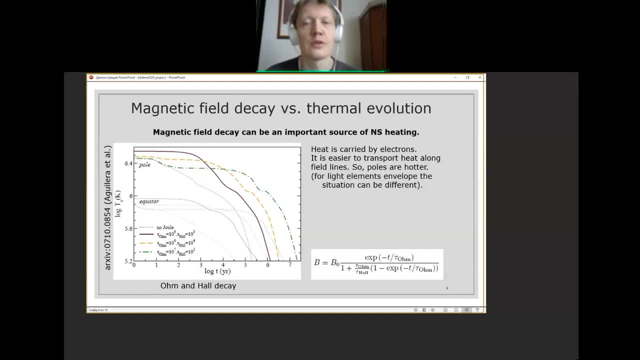 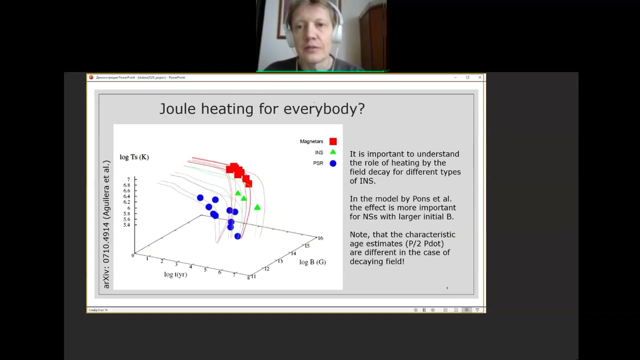 internal parts of neutron stars. Internal parts of neutron stars are mainly important, even not to astronomy but to nuclear physics. So in this respect, really, telescopes work as addition, important addition to accelerators. So if- and this is, I would say, an effect- 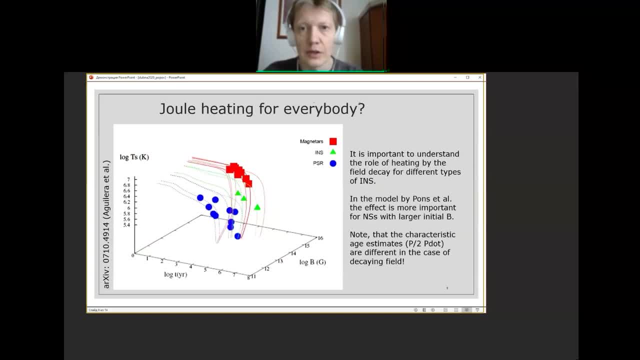 if strong magnetic field evolves faster, it contributes more to heating of the crust. then this effect is more pronounced in magnetars. Indeed, we see it. And here, in this more 3D plot, the authors of the plot try to put together: 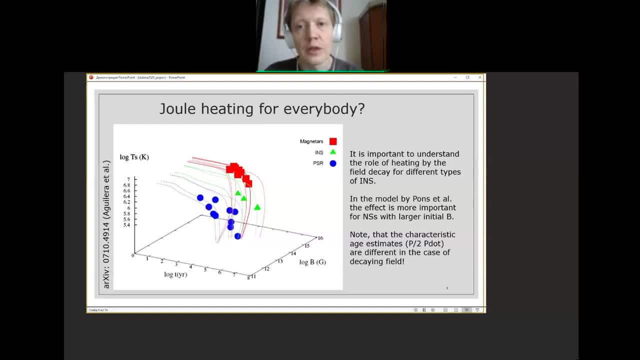 thermal evolution and thermal evolution. magnetic field evolution and magnetic field evolution somehow unfolds, as I told you. period evolution, So normal radio pulsar sources with surface poloidal dipoles or magnetic field 10 to 12 Gauss. they do not feel significant effect. 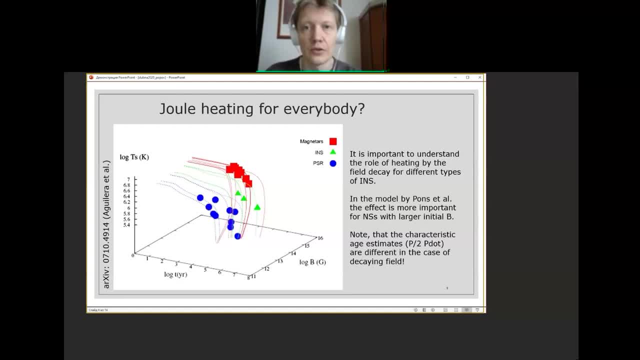 of magnetic field decay, at least in terms of the thermal evolution. But for magnetars the effect is more important And isolated, cooling. neutron stars, the Magnificent Seven sources, for example, they are in the intermediate situation, Also when people started actively. 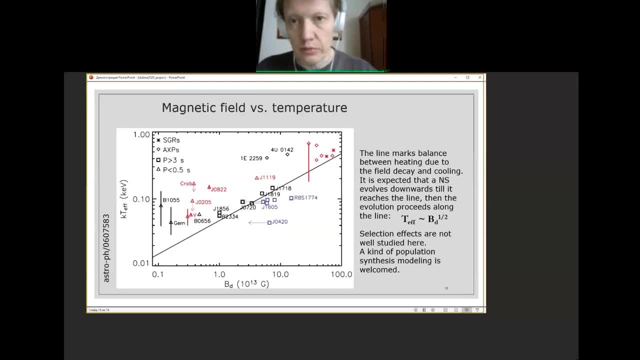 to work in the field. it's all you see. it's, of course, 21st century science, just not say last year science. And they discovered a very interesting feature, which is illustrated in this nice plot On the vertical axis. 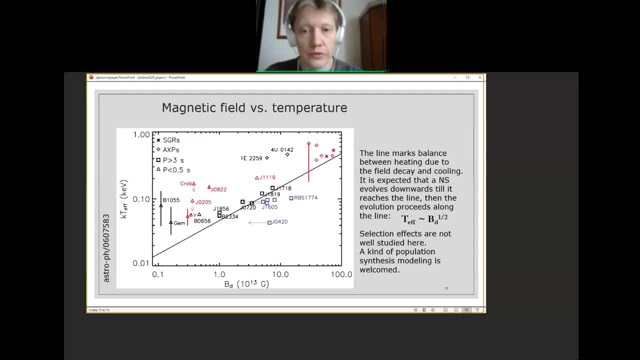 we have effective temperature of the neutron star surface And you see it's in the X-ray range And on the horizontal axis, dipole magnetic field. What is this diagonal black line? It shows a very interesting feature Imagine we have in the beginning. 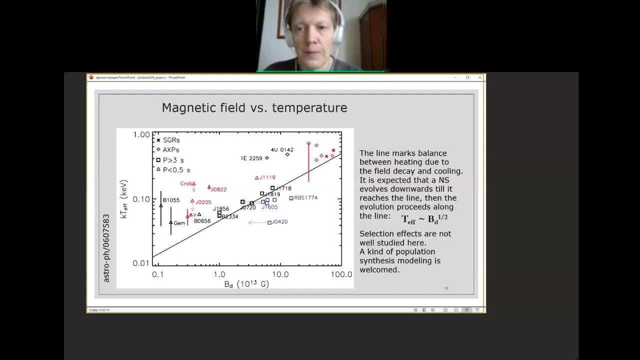 a very hot neutron star. This is normal. Then it starts to cool down due to neutrino losses from its interiors And so on. this plot: a neutron star rapidly moves down, It moves down, It moves down, But at some moment. 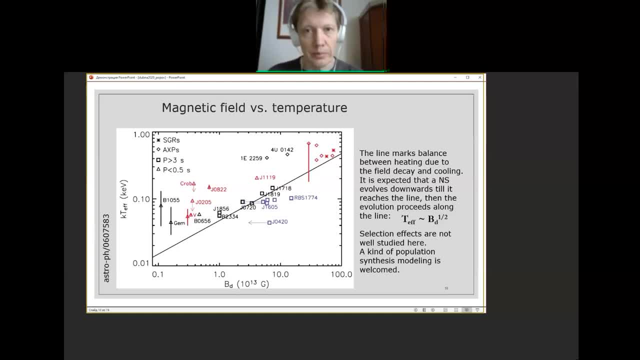 it stops to cool down rapidly because now it reaches its surface. of course, while speaking about the surface temperature, Its surface reaches some minimal temperature And this temperature can be supported for a relatively long time by magnetic field decay, by additional heating due to magnetic field decay. 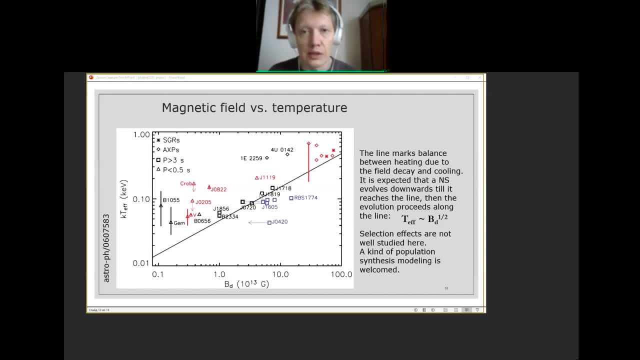 And so then a neutron star will start to move along this line. Of course such a line depends on exact internal properties of the particular neutron star. So there is no universal line. The line can be plotted for a given neutron star, But neutron stars. 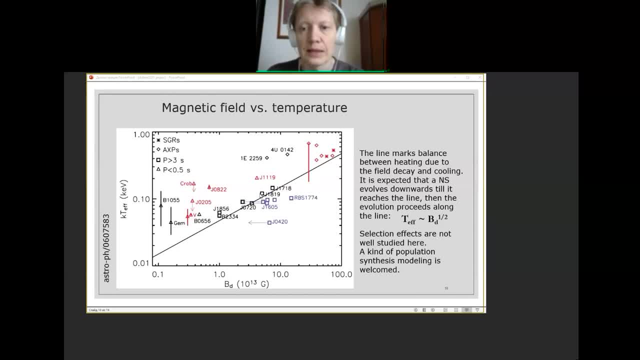 are not much different one from another. So it is relatively narrow, I would say band, not of course infinitely thin line, but relatively narrow band which can successfully describe the general observational appearance of neutron stars of different kind, And this plot clearly illustrates. 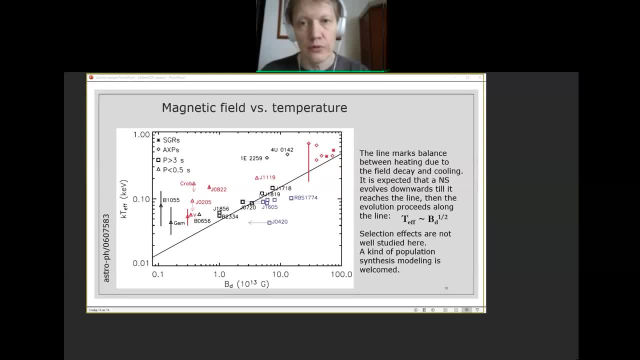 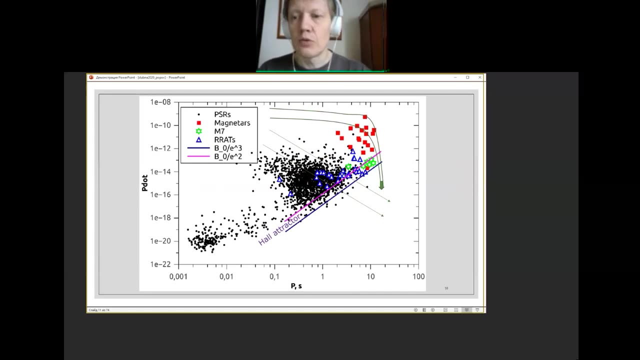 that magnetic field decay is important for many types of neutron stars, not only to those observed as magnetars. So let me come back to the PP-dot diagram and draw another line. So again, PP-dot diagram: different types of sources: radio pulsars. 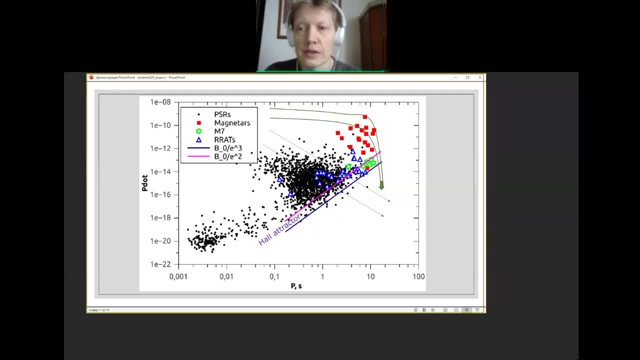 magnetars, Magnificent 7, rotating radio transients, evolutionary tracks, as we discussed already. for magnetars, magnetic field decay is important And so they turn down, moving generally to the right. they turn down Because of rapid magnetic field decay. 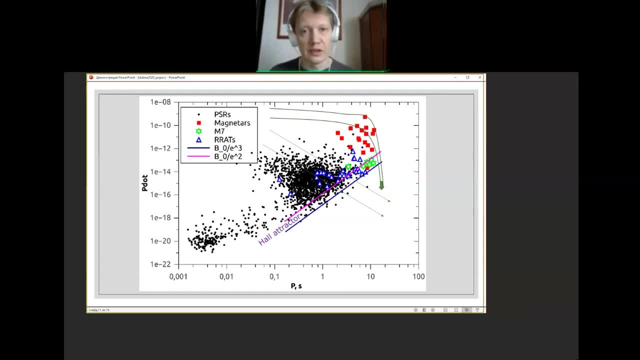 radio pulsars do not feel strong magnetic field decay. Still, I will come later to the point that they feel some magnetic field decay, at least during some periods of their life. And then I plot another two lines which will be important for us later. 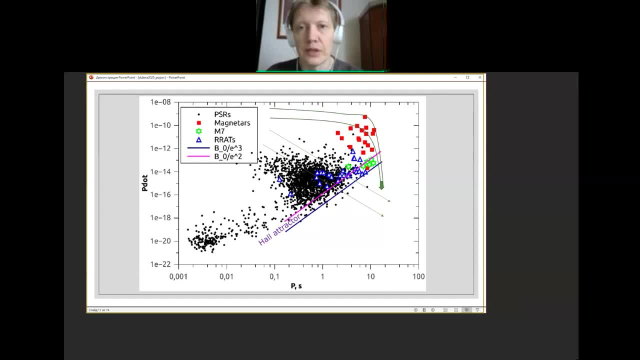 This is a very interesting stage, theoretically predicted six years ago, six, seven years ago- due to very sophisticated numerical modeling of magnetic field evolution, And this stage is called the Hall attractor. This is quite an interesting feature. It's related to 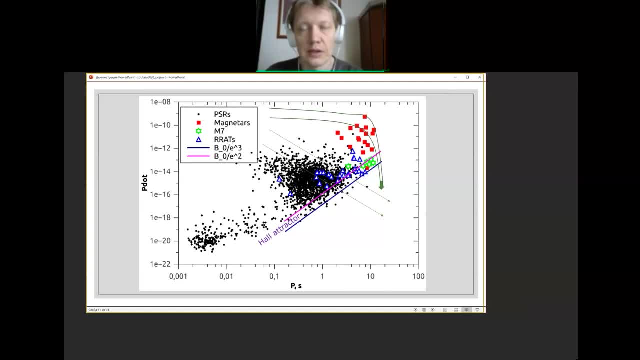 evolution of topology of magnetic field inside the neutron star. Initially it was obtained for crustal models, but then it was also confirmed in models which takes into account the magnetic field in the core And at this, since this stage is reached, the rapid magnetic field evolution. 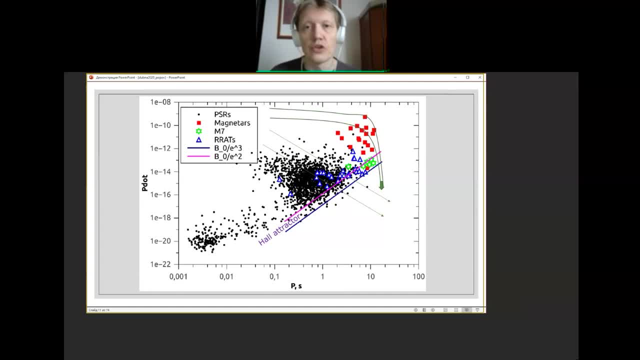 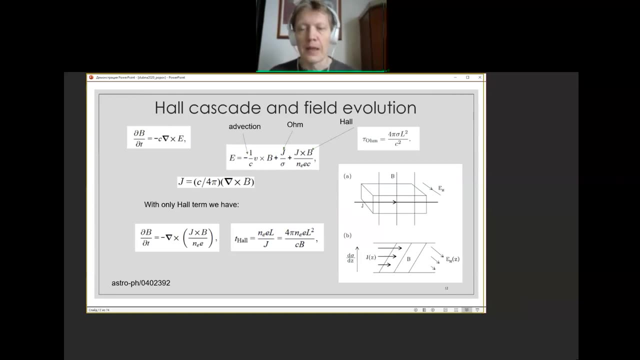 is stopped. This is quite an important feature. It would be nice to see it in observations, maybe very close to it, but still we do not see this stage in neutron star evolution. So OK, let's come to formulas finally. So astrophysics is not only. 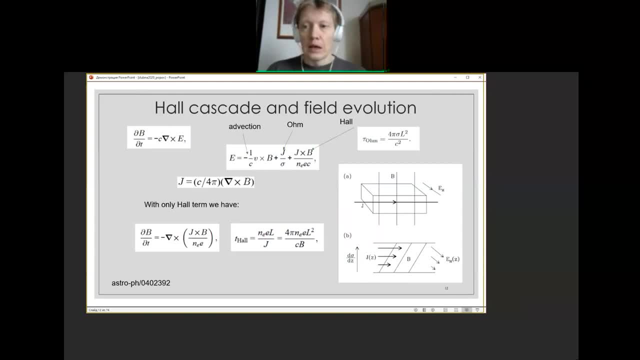 beautiful pictures. So we have to describe magnetic field evolution And if you are interested in the subject, I strongly recommend the paper by Cumming and co-authors. Mainly, I refer to papers by their archive numbers, not by journals and years. 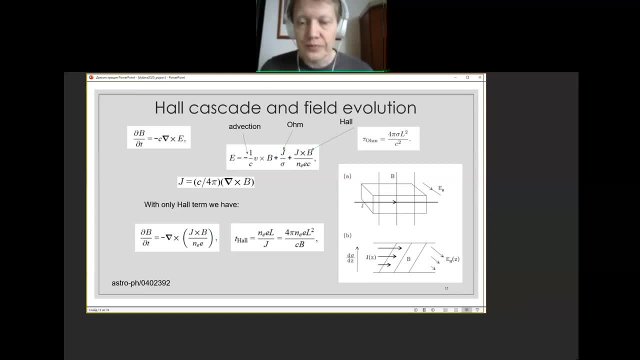 since it's just easier to find the paper in the archive. So mainly you'll see numbers referring to the archive. So in the magnetic field evolution we have quite a simple equation. Of course, to put it in exact physical picture: inside the neutron star. 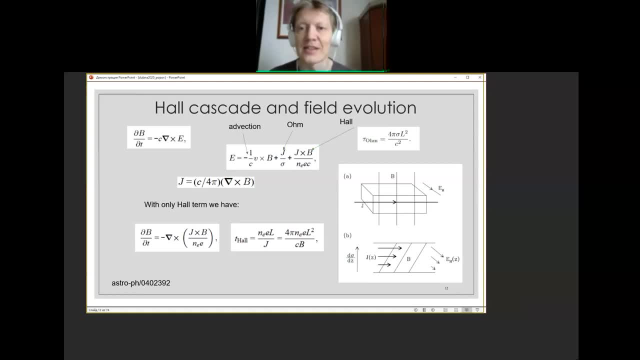 is not a trivial task. But for initial analysis the equation is not that difficult And we have two main contributions to magnetic field evolution, So omic evolution and whole evolution. Whole evolution is illustrated in the plot on the right. Whole evolution is not. 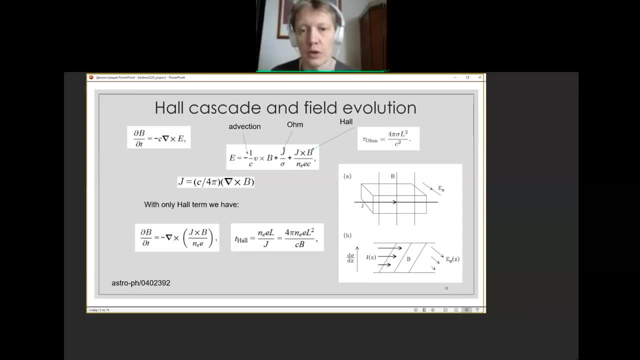 a dissipative process. So this whole cascade is not a dissipative process In the crust. it is related to the fact that electric currents are different at different depths inside the crust because conditions are significantly changing. Electronic concentration is changing. It's growing down. 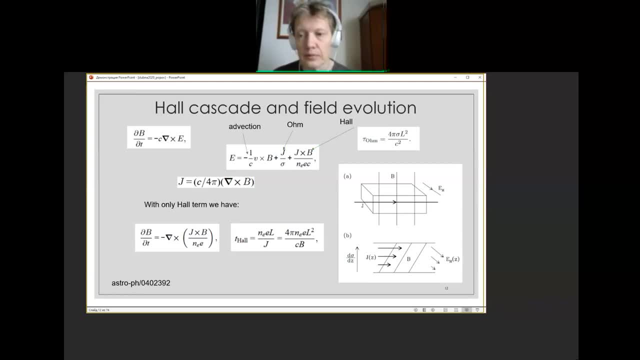 And so currents are different And because of that the topology of magnetic fields, of the magnetic fields, starts to change. It is modified, And this modification goes in mainly in one way. It works more or less like turbulence: Large scale magnetic field. 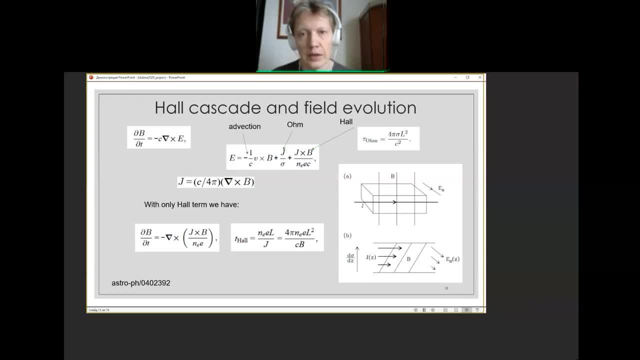 is converted into small scale magnetic field. Again, dissipation is not happening during this process. But since you put magnetic field at smaller scales, then omic dissipation becomes much more important, because omic timescale- here it is shown- is proportional to the scale. 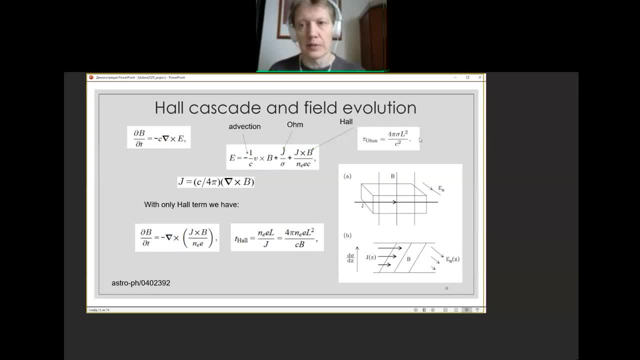 of the field square. So since this scale becomes smaller, characteristic timescale for the omic dissipation becomes smaller and magnetic fields decay rapidly. So if you have an effective process of modifying the structure of the magnetic field, it is more important. Omic dissipation is always ready. 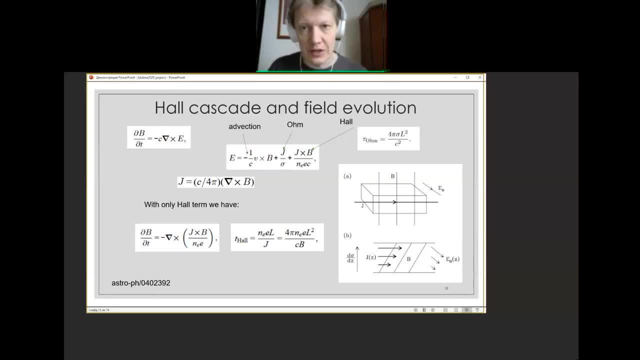 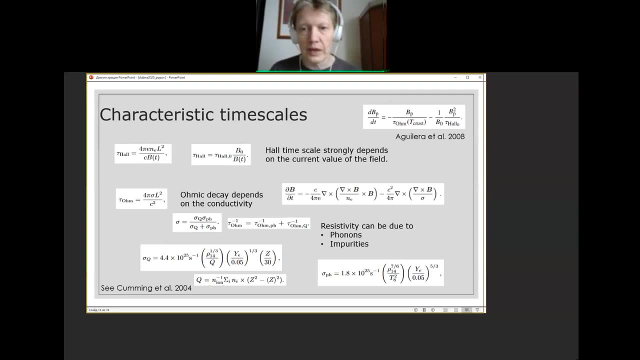 to produce magnetic field decay if you can make the characteristic timescale small. So we can define these two timescales: the whole timescale and the omic timescale. For the whole timescale, it is important to note that it is inversely proportional. to the magnetic field itself. This means that this timescale is smaller for large magnetic field and because of this, mainly magnetars are evolving so rapidly. So it's not that omic dissipation by itself due to resistivity is more efficient in magnetars. 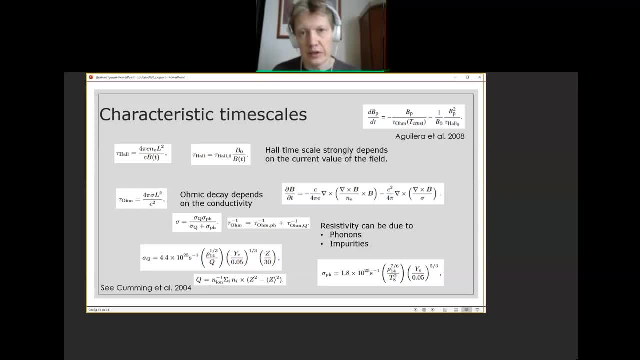 It's important that the whole cascade is very effective in magnetars. So magnetic field is quickly driven to small partial scales and then the omic dissipation starts to be very effective. So omic dissipation by itself can be divided in two parts. 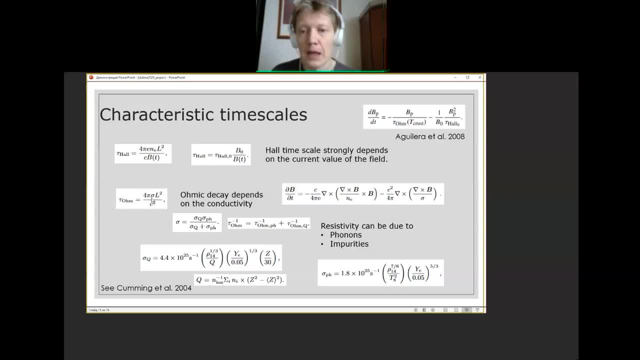 So here we have conductivity, sigma and this. so the resistivity is mainly due to two different processes. So the first one is scattering of electrons, of phonons. So since crust of the neutron star is hot, the interaction between electrons and phonons is very effective. 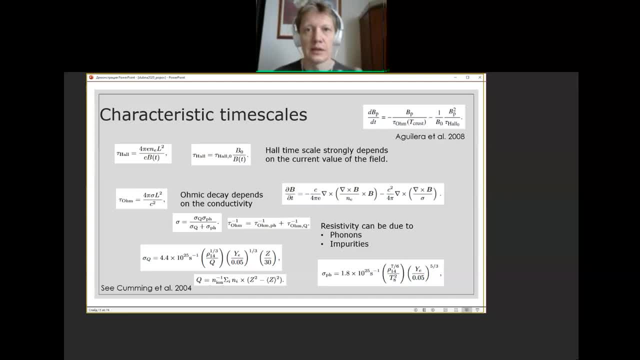 and it results in significant resistivity. So currents are rapidly going down, and so the magnetic field is going down. We have a rapid magnetic field decay because of phonons, and this process is going on till the neutron star is hot. So here we see. 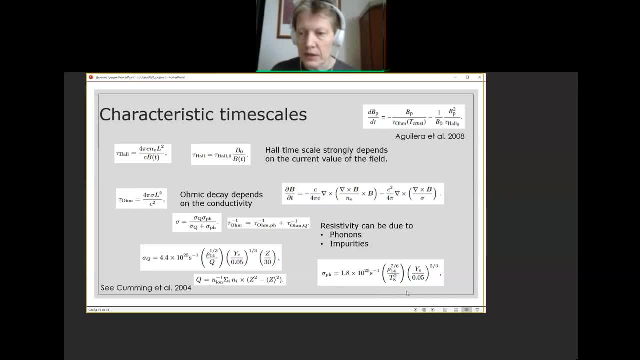 the conductivity and temperature is here. So for high temperature we have low conductivity. Okay, The second process is, I would say, more normal. There are impurities in the crust and electrons can scatter off this defects, these impurities in the crust and this. 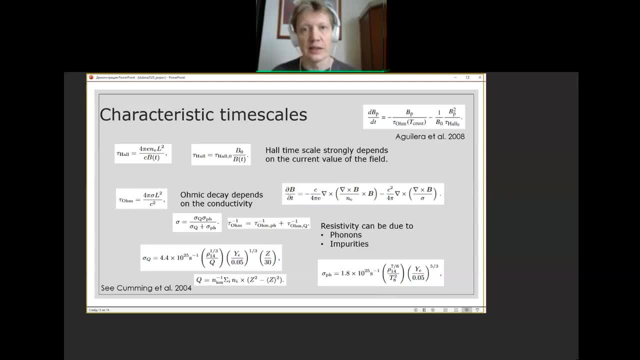 process is not temperature dependent, It just depends on properties of the crust. So this, this parameter depends on the depth inside the crust, because it depends on concentration of electrons, on the amount of impurities, on nuclear composition, which all these parameters are rapidly changing. 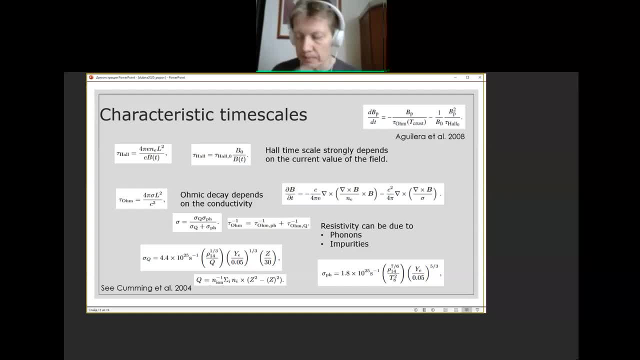 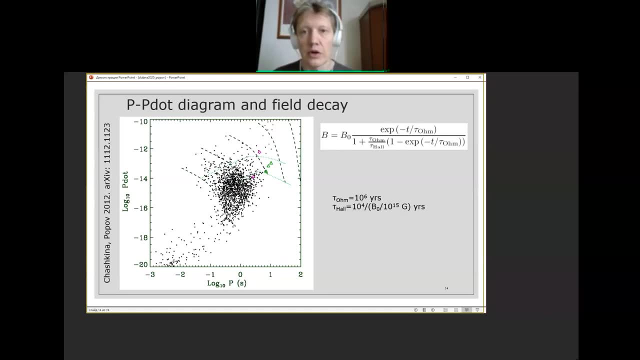 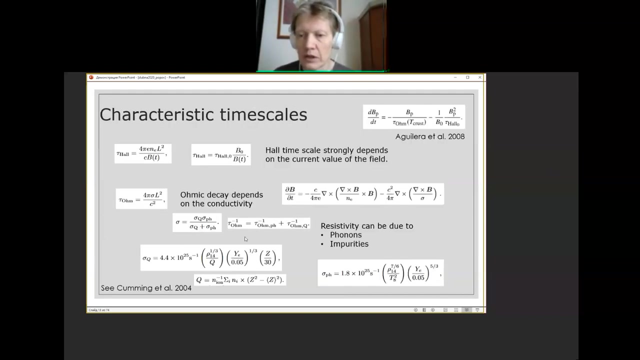 with depths in in the neutron star. Okay, So if we make a simple model described by two processes: hole and whole cascade with its characteristic time scale, tau hole and ohmic dissipation with another characteristic time scale, maybe I want to underline here that of course 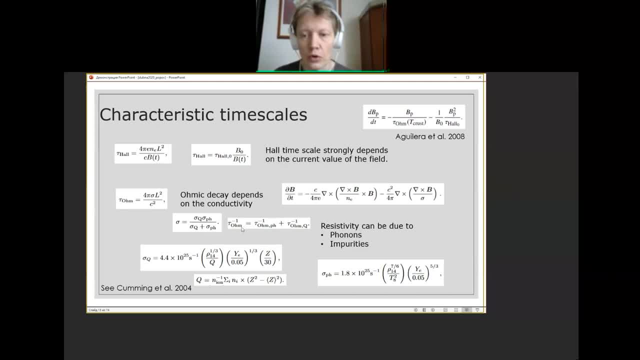 there is a very simple equation for for the total ohmic time scale, which is, which is defined by sum of inverse time scales for ohmic dissipation on phonons and impurities. Okay, So if we make such a simple model, we can write simple equations. 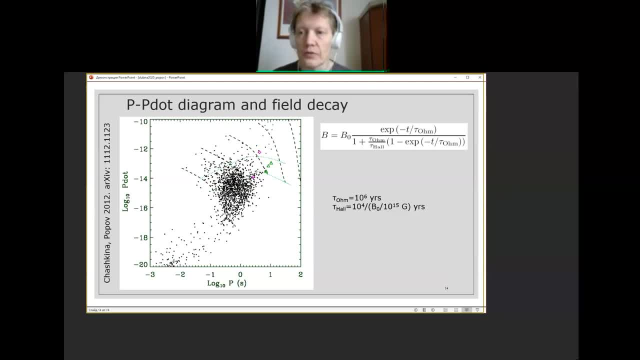 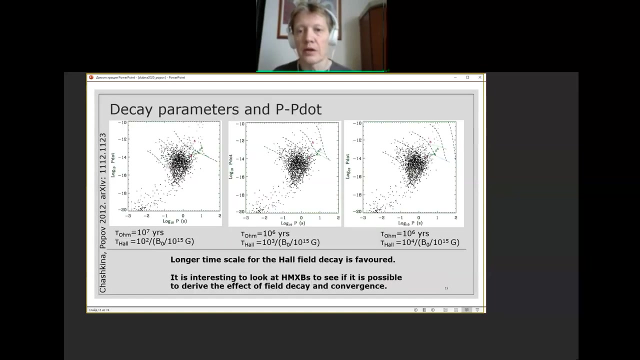 and there is a solution for such an equation and we can plot simple lines on the pp-dot diagram, just varying two parameters, these two characteristic time scales and, of course, playing with initial magnetic fields. Even in the framework of such simple model, we can make some conclusions. 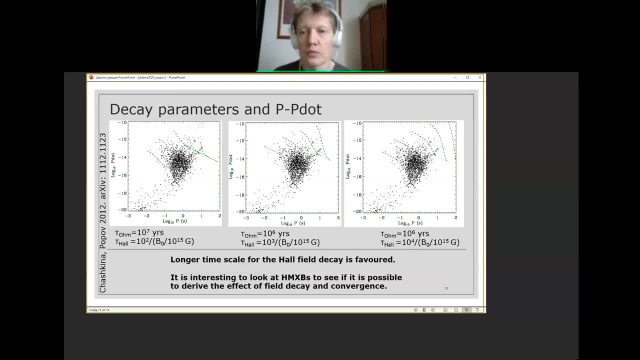 so let's vary these parameters and we'll see, for example, that for some set of parameters you see rapid convergence of evolutionary tracks, and if this would be the case then we would observe pile up of sources close to this line. it's not happening, so most probably. 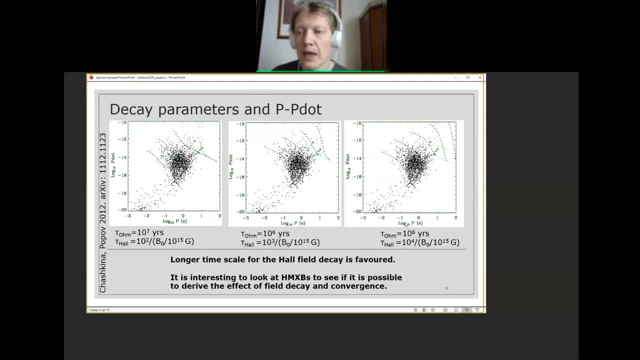 something like this situation happened and we can have some guess. because we are talking about the simplified model, we can have a guess of these parameters, how they depend on what are typical numbers and how they depend on some internal parameters of neutron stars we can try to make. 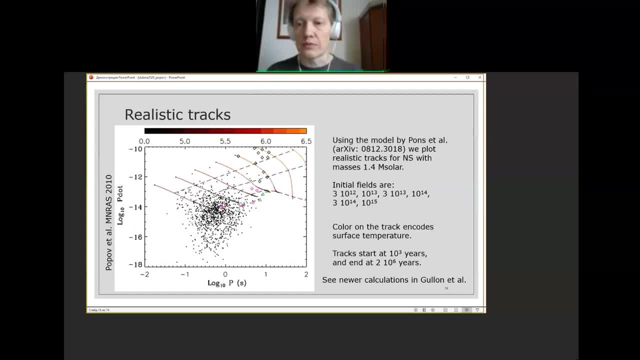 more detailed calculations, and that we did with colleagues from Spain which actually had the, the microphysical model for the magnetic field evolution, and we added the astrophysical part for it and we'll see here, in addition to rotational evolution, in addition to magnetic field evolution, also thermal evolution. 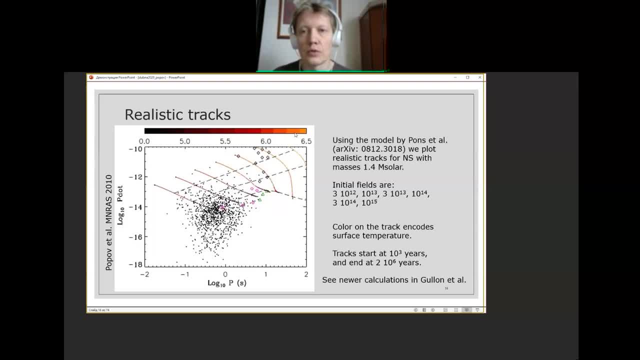 because this color on top encodes temperature of effective temperature of neutron star surface and this is just a logarithm of temperature. so six is one million degree and we see especially on this track how, starting from yellow orange, we come to red and dark red, finally this dark red. 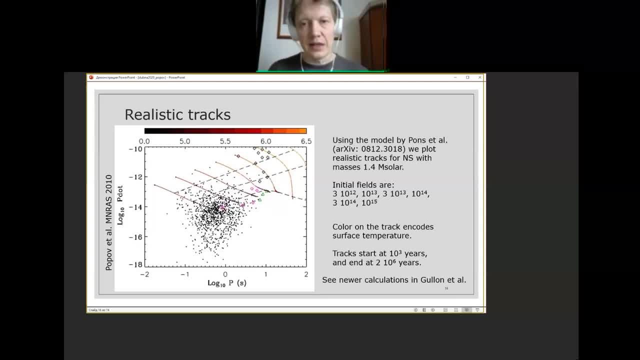 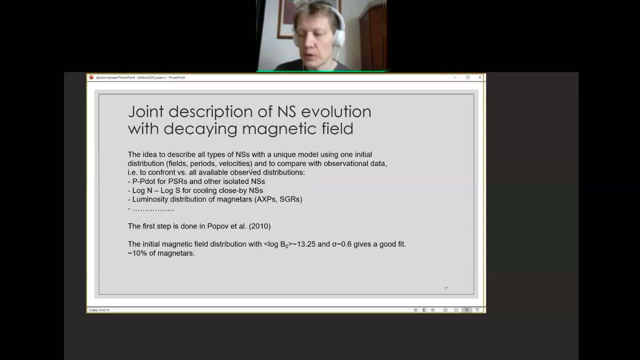 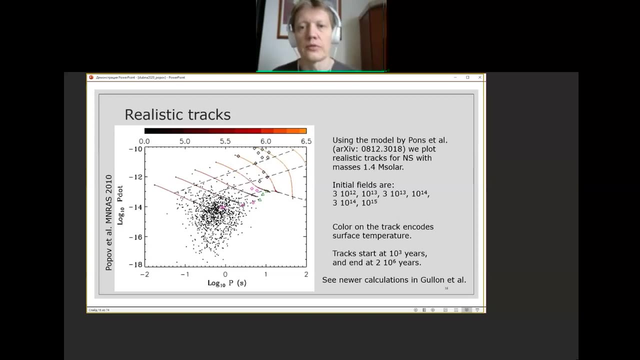 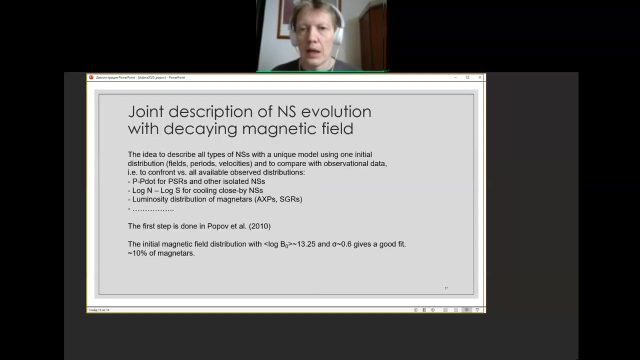 because the magnetic field decay stops here. so in this part of curves here, here, here, magnetic field decay heats up the external part of neutron star and when you slowly switch off the magnetic field decay, the temperature goes down. so it goes down not so fast, but it goes. 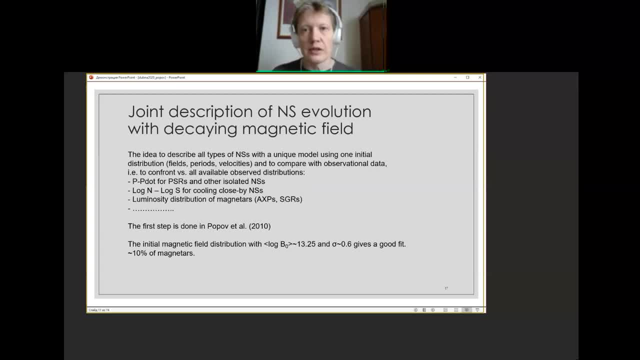 down. so in this framework, in this approach, we try to model different populations of neutron stars, to describe them in one general picture, and the idea is not actually that direct not to make this picture, but then you try to put it in a general physical picture in the 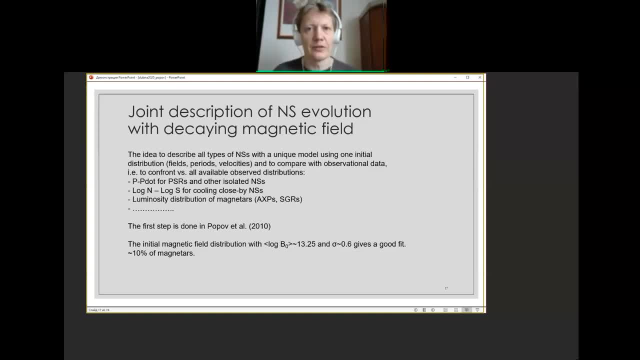 general physical model. you have much more constraints on parameters of this model because otherwise you nearly have like everything is possible. but when you take many of these things and you have a very large number of neutron stars, you have a very large number of neutron stars, so you 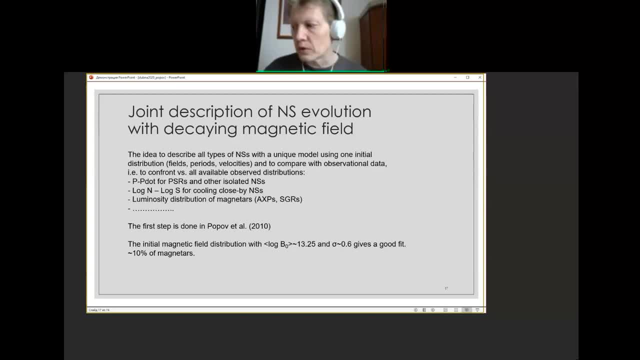 have a very large number of neutron stars and you have a very large number of neutron stars and you have a very large number of neutron stars and you can take a lot of the magnetars and you can take a lot of neutron stars and you can take 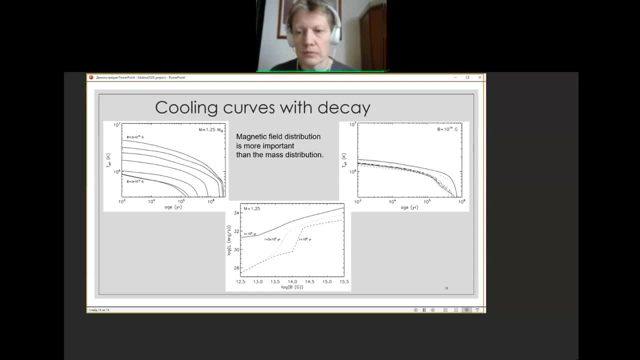 a lot of magnetars and you can take a lot of neutron stars and you can take a lot of magnetars and you can take a lot of neutron stars and you can take a lot of magnetars and you can take a right. we fix magnetic field at relatively high level and we vary neutron star masses and we have 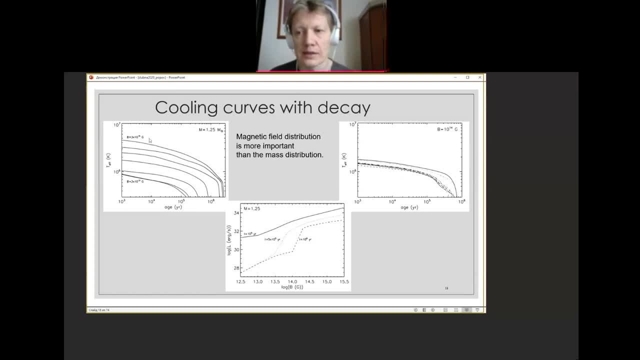 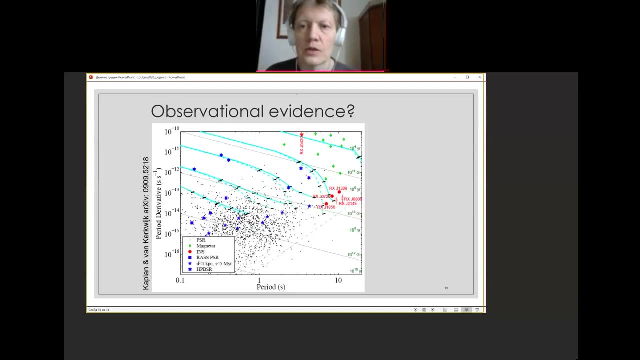 some difference in temperature evolution, but it's not as large as it is here. so for magnetars, indeed, magnetic field evolution is the main driver. i just wanted to illustrate it here. just before, or actually when we finished our paper, observers started to say that actually they need something. 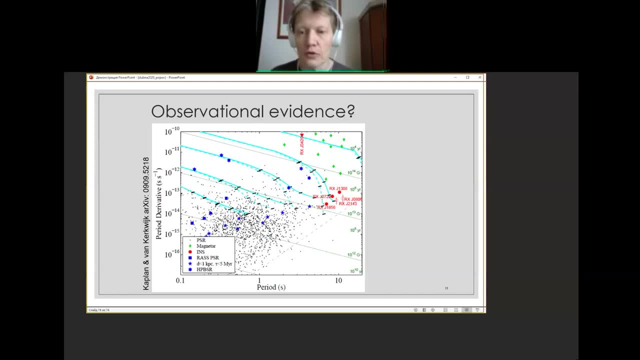 like this. this is a plot from 100 percent observational paper and these blue lines actually what observers wanted to have: how they see, how they foresee evolution of magnetic field. and it was quite nice that at the same moment- absolutely independently because we worked in parallel with these authors- we came to similar conclusion about general properties. 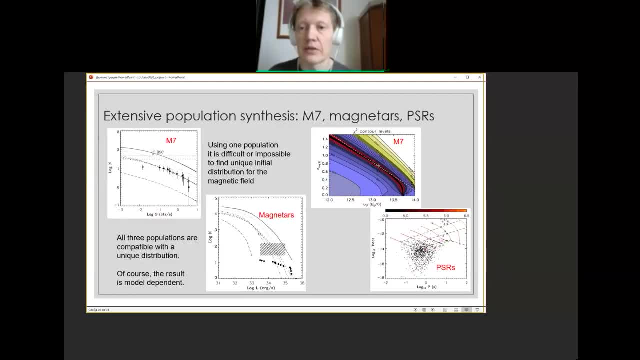 of magnetic field evolution. so, okay, we explained three population of neutron stars in one framework. that was quite fine. and, what is important, the magnetic field evolution was the, the main ingredient of this model. it was, uh, very important for magnetars. it was somehow important for the magnificent seven who are actually the center of the magnetic field evolution, of the magnetic field evolution. 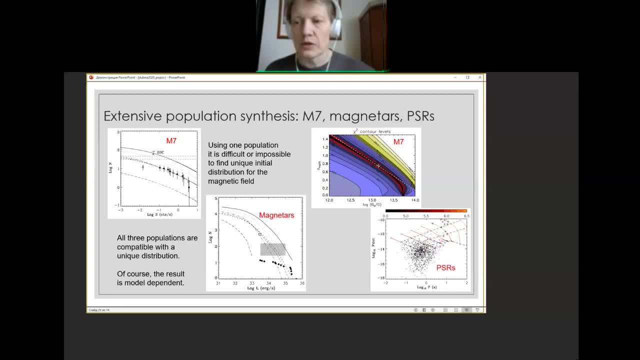 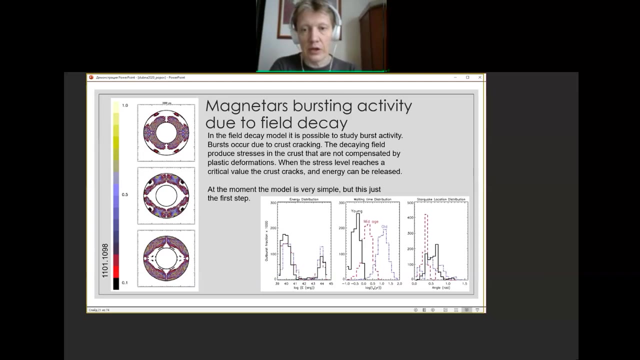 of the magnetic field evolution and uh. magnetic field evolution is much less important for radio pulsars but we get better fits if we include magnetic field evolution, long-term magnetic field evolution, going all the way. with the same physics, people start studied several other aspects of magnetic field evolution. i think i have to speed up a little bit. so there are many interesting. 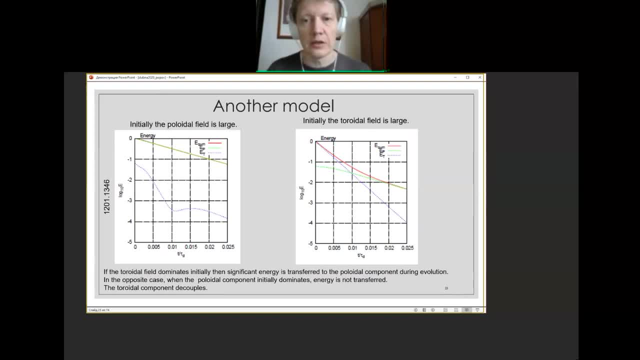 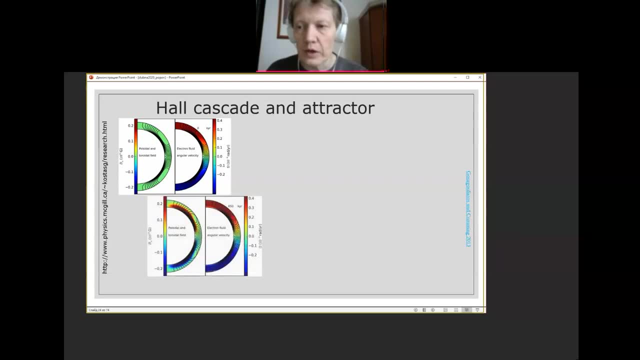 modeling during last years about the magnetic field evolution and the crust. so i want to come to this point um where, uh, the authors found for the first time this whole attractor. so they calculated magnetic field evolution and the crust and they found out that um evolution starting with different initial conditions, finally come to some stable 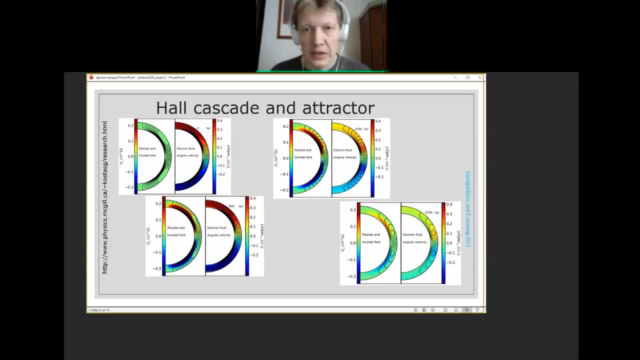 configuration at which the whole cascade is stopped. this is quite interesting because it has important astrophysical predictions. uh, this rapid episode of whole evolution is stopped not just because the magnetic field, which is in denominators, you remember, in the time scale, becomes too small, so the time scale is too large. it stops earlier because the magnetic field finds: 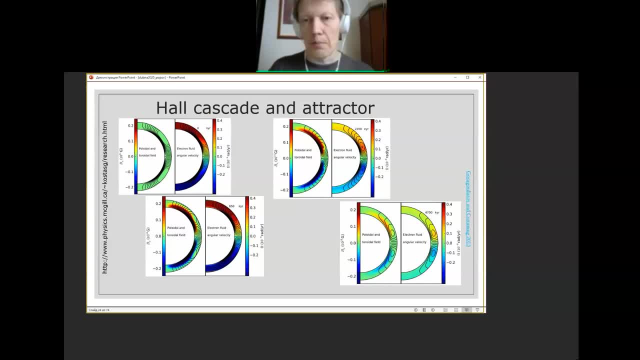 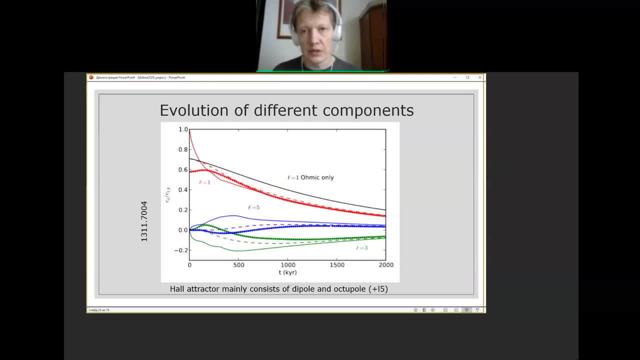 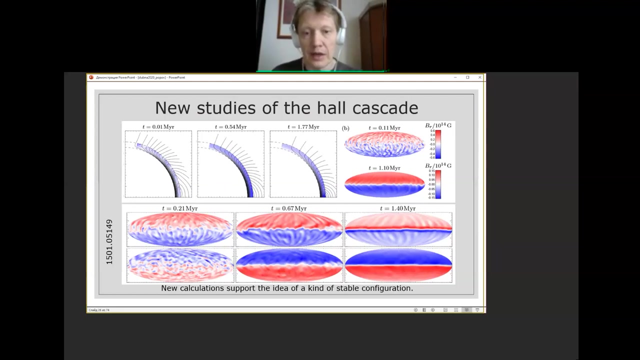 some structure which makes it stable against the rapid whole cascade. this is quite interesting and the authors even predicted. of course, now it depends on some details in the model predicted, the structure of external magnetic field corresponding to the whole attractive. so it's a mixture of uh. mainly it's a mixture of dipole and octopole. it was independently confirmed. 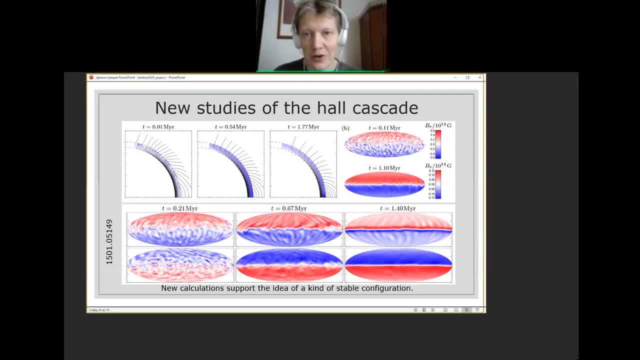 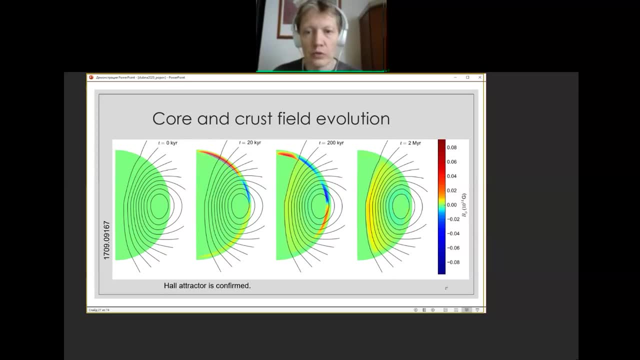 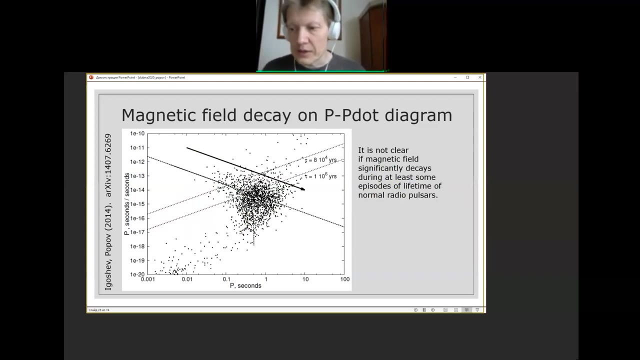 by several other studies. so just believe me, there are calculations and nice pictures about it. it was confirmed uh with um, with a model which included uh field in the core. okay, so let's put it aside and uh, come to the next uh step. but of course we will come back. we'll remember what we. 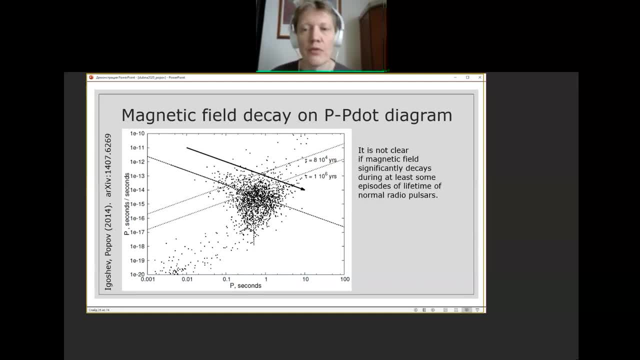 said before. uh, let's come into observations. for quite a long time people started to, people tried. quite a long time ago people started and for quite a long time they tried to um find direct observational evidence for magnetic field decay in normal radio pulses, and results were quite controversial. um, if we speak about modern modeling model, 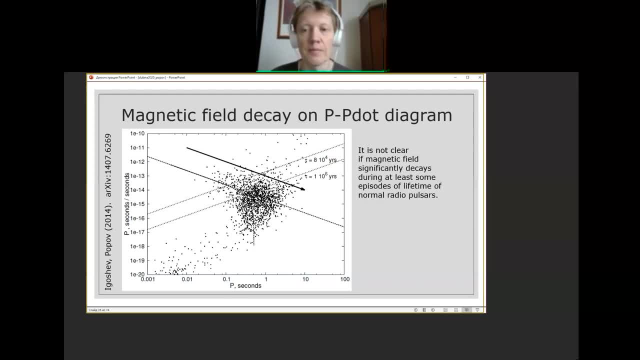 modern calculations then? um, at first it's necessary to say that definitely there is no significant long-term magnetic field decay in radio pulses, on and on. on the other hand, it's quite obvious that if you add an additional parameter in your model magnetic field decay, you obtain a better fit. so it looked like as i showed you before, as 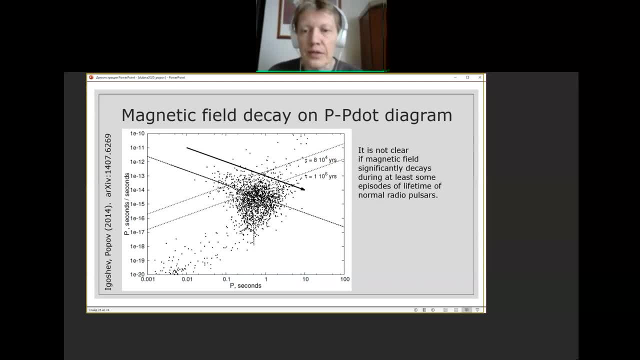 also, we got in our model that very moderate field decay in radio pulses fits a little bit better. but is it the end of the story? maybe not. and um, some time ago andrei goshev suggested another method how to probe magnetic field evolution in relatively young, i would say middle- age. radio pulsars, middle agent, logarithmic scale. 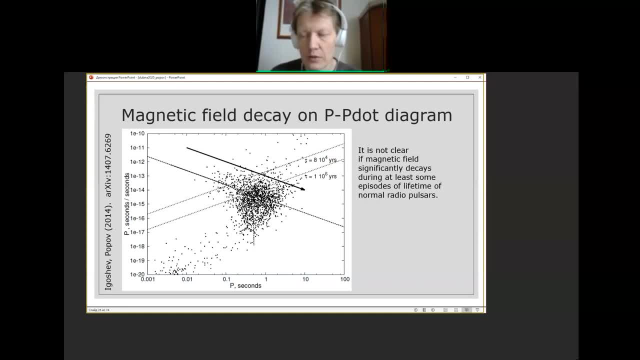 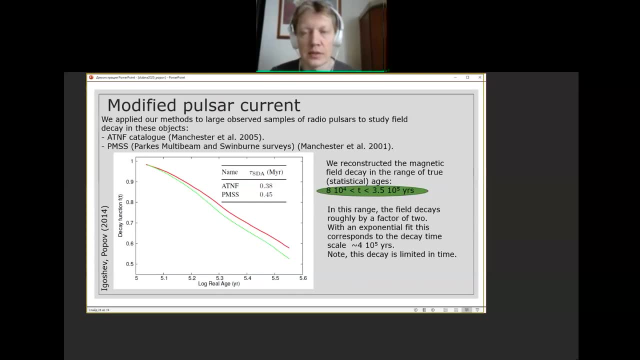 radio pulsars and uh, we got quite surprising results. we started radio pulses with ages significantly less than one million year, so we were limited by ages about 400 000 years, and we obtained that during several hundred thousand years magnetic field in these objects experience field decay. so on the plot, the field. 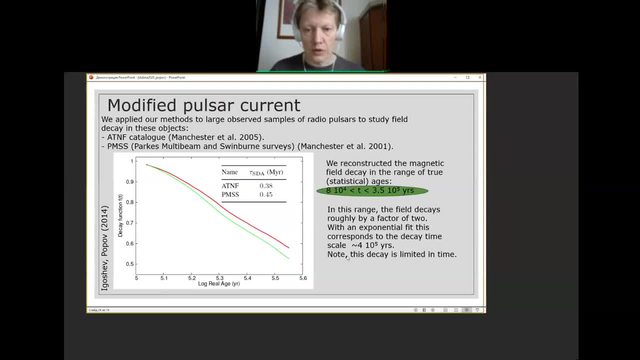 is normalized to its initial value. so this 0.5 means that the field decays by by factor two. so if you continue this magnetic decay for the whole lifetime of a radio pulsars, of a radio pulsar, you are in trouble. it's absolutely impossible, because this is a 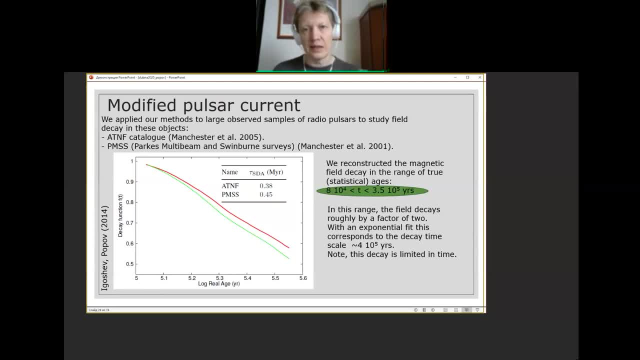 very rapid decay. so on one hand, we see some evidence for field decaying young pulsars. on other hand, we need a mechanism to switch it off because it cannot last for long or, of course, we are wrong with our models and there was nothing to switch off. 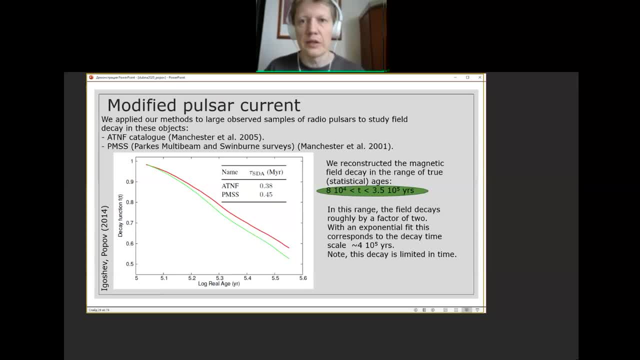 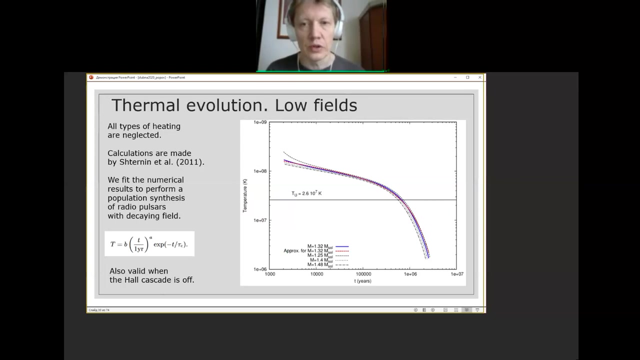 Still we think, and we repeated these calculations and confirmed our results. We think that this episode of magnetic field decay is real. It's obtained on a large sample of large uniform amounts, a sample of radio pulsars, And then we tried to study the situation in more detail. 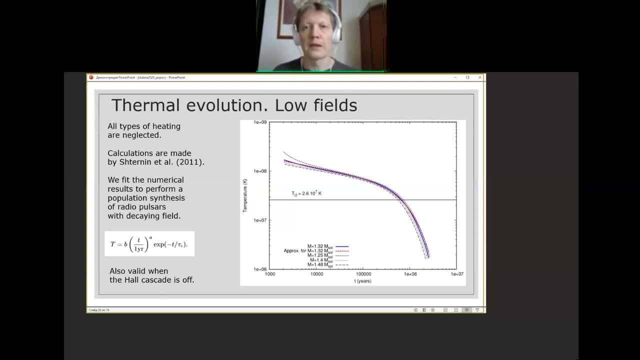 We started to model the magnetic field evolution in young neutron stars And, as you saw, significant decay, significant contribution to the only magnetic field. decay is due to scattering of phonons And this process depends on the thermal evolution of neutron stars. So we tried to look at it in more detail. 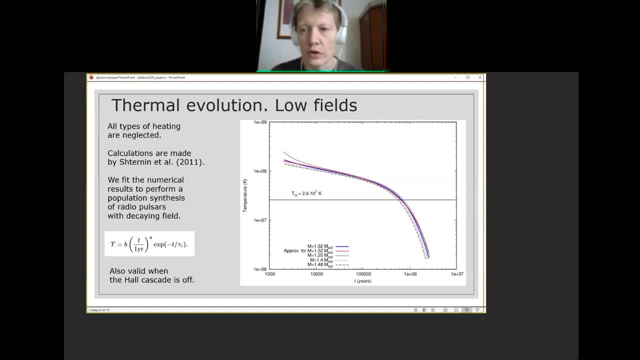 People from Yofi Institute provided us with cooling curves, which you see in this plot. So these are calculations by Peter Stern and his co-authors. We found a good analytical fit for internal temperature, So not for the surface, but for internal temperature of a neutron star. 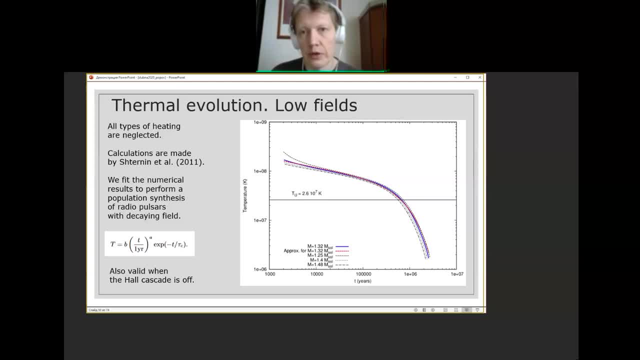 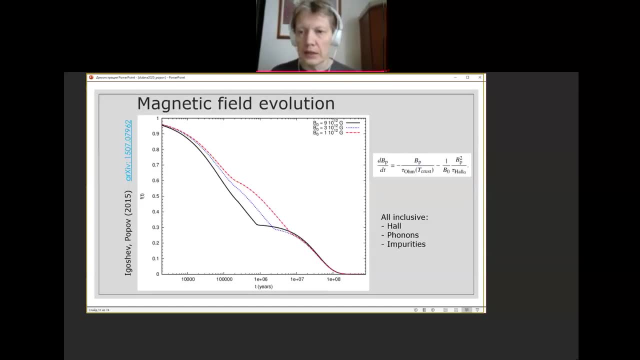 And we implemented this thermal evolution into our models of magnetorotational evolution. And what we obtained? these are plots of magnetic field evolution. Again, the field is normalized to its initial value. Three values of magnetic field typical for radio pulsars are used here. 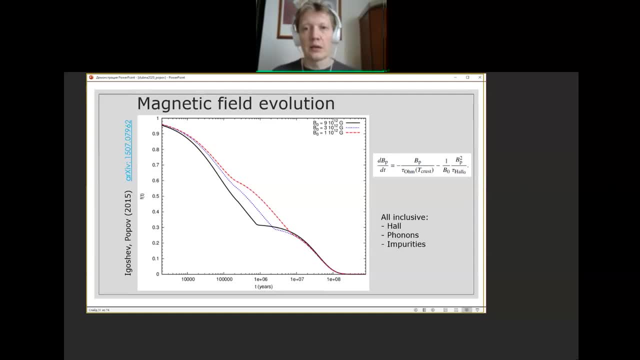 And we included the whole cascade: ohmic decay due to phonons, the ohmic decay due to impurities. Of course we see that larger magnetic field decays, decay more rapidly. So in say, less than one million year. 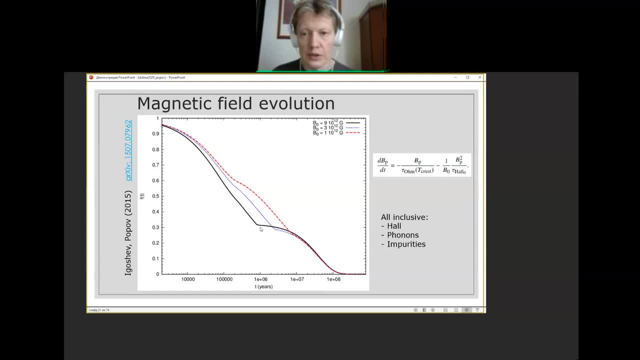 large magnetic field decays by two-thirds and the smaller magnetic field just by one-third roughly, Or maybe one-half in the same period. And, what is important, we can not switch off, of course, the decay completely, but we can significantly increase. 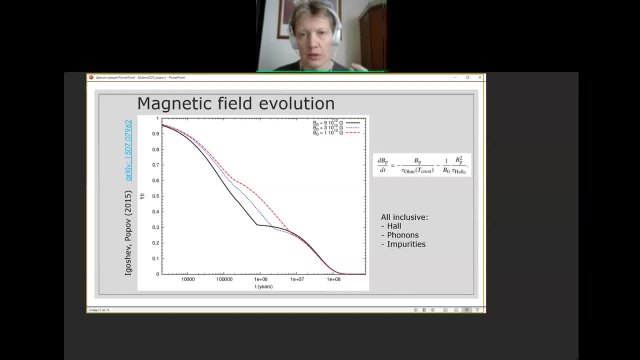 the time scale of magnetic field evolution, because neutron stars are rapidly cooling down, So phonons are not effective anymore and so magnetic field starts to decay slowly because resistivity goes down and at later times. later times means a few hundred thousand years. 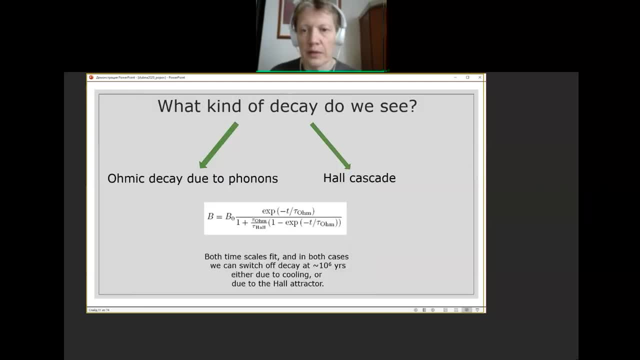 resistivity is determined just by impurity. However, to come to this conclusion, we made some additional studies Because it was not obvious. we suspected that maybe it's not just cooling which switch off the decay in radio pulsars, but maybe it's whole cascade. 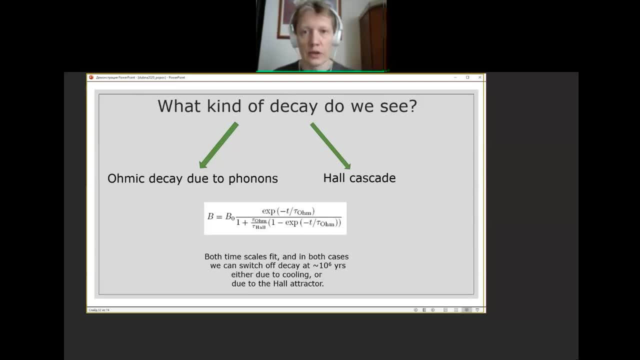 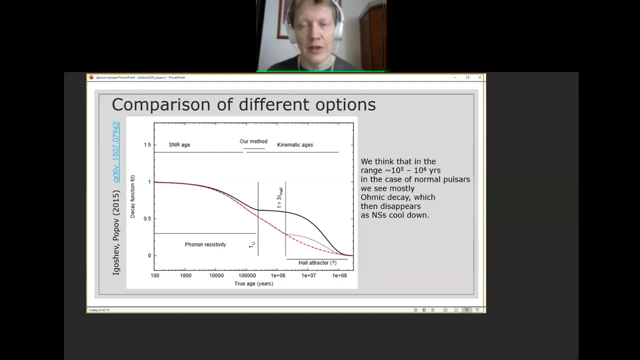 which is stopped because of whole attractor. So it was very attractive to find whole attractor in normal radio pulsars. So we couldn't stand this temptation and we started it. Unfortunately, we came to the conclusion that no, we don't see this very nice effect. 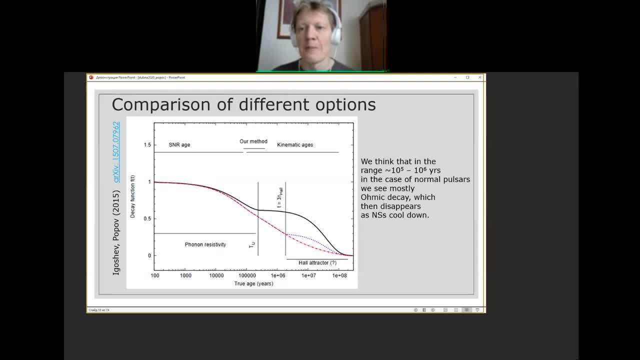 which nobody yet saw in observations. So we also failed. But what we see? we see the effect of cooling, So some critical temperature is reached. Here it is. Of course it's a sketch for different neutron stars with different masses, different equation of state. 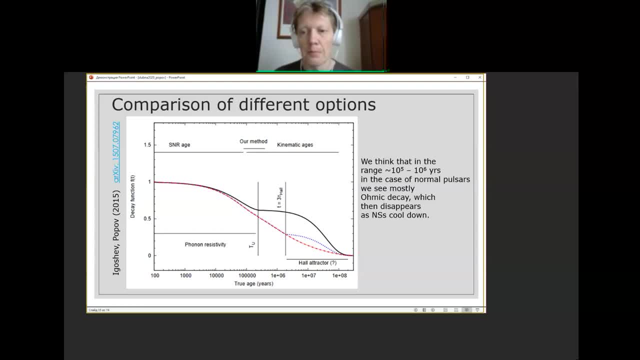 Lines will move slightly on this plot, but characteristic time scales would be of the same order. So it looks like we found an evidence for an episode of magnetic field decay in young radio pulsars because of phonons, And then this magnetic field decay is switched off. 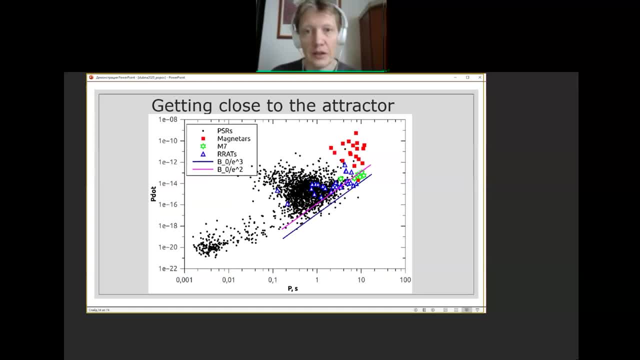 Still, we wanted to find attractor and we made another attempt. So you remember these two lines. they roughly correspond to the whole attractor And it would be nice to find neutron stars close to the attractor and to find some particular features. 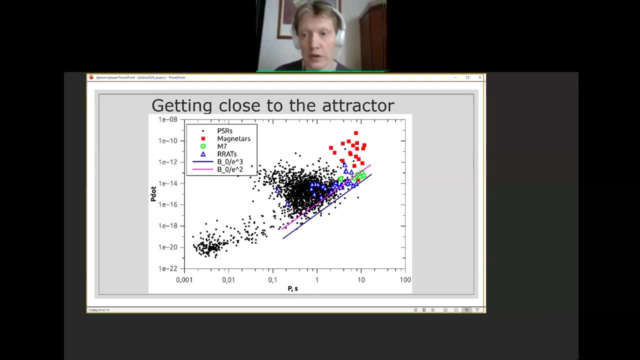 of the sources which would correspond to the attractor. So we focused on the Magnificent Seven. They are shown in green here, Magnificent Seven: they are thermally meeting neutron stars And the map of temperature, the thermal map of a neutron star. 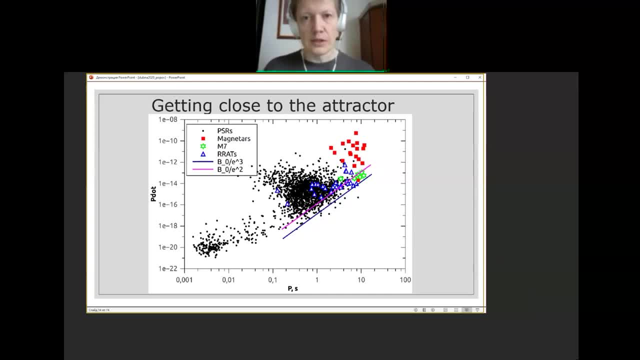 depends on the magnetic field, Because heat transport in the outer layers depends on the magnetic field. Heat is transported by electrons, as I told you, And electrons, of course, like to move along magnetic field lines, So they easily move along field lines. 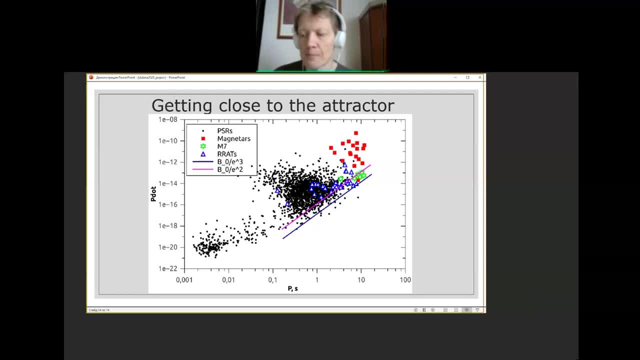 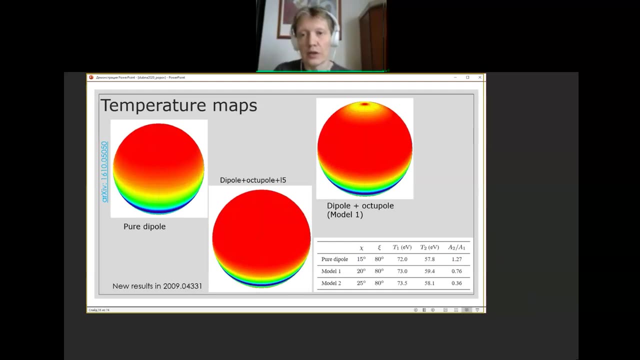 and they don't like to move perpendicular or to the lines, And so temperature map depends on the magnetic field structure, Because magnetic field in some sense channel heat to the surface, And with Italian colleagues we calculated maps for different configurations of the magnetic field. 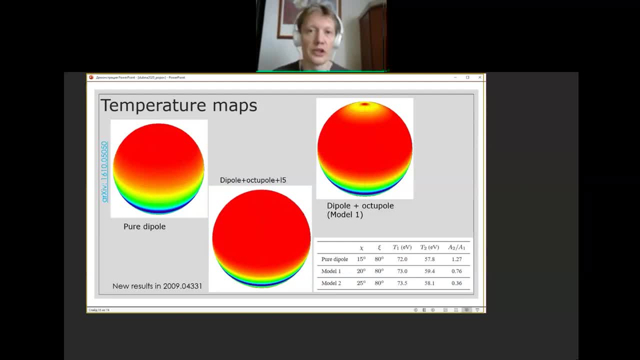 including the model which corresponds to predictions of the whole attractor. So that was the first step. We made it four years ago And then we applied it to one the best study of neutron star of this kind, to the source RXG 1856.. 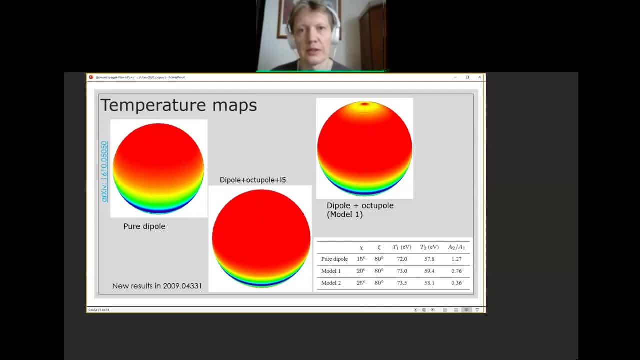 And we unfortunately didn't find that the prediction made with the whole attractor fits the data. But very recently, in September this year, Italian colleagues with a new PhD student significantly enhanced, advanced these calculations And it seems that maybe they will be able to see. 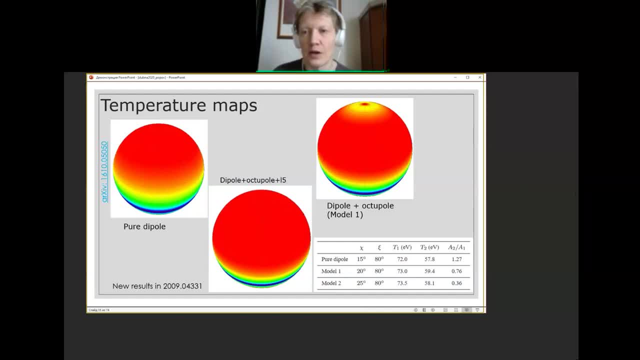 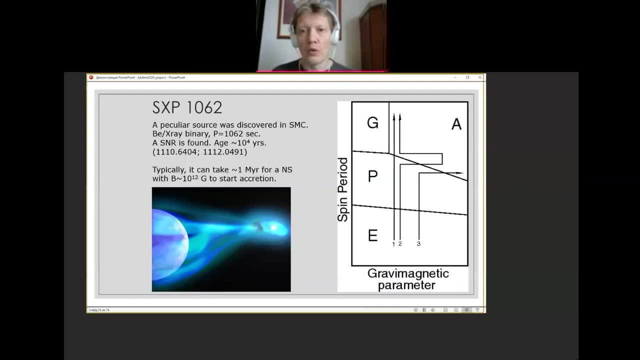 whole attractor in these neutron stars. So I hope very much that in one, two years these results will be out Okay. Where else do we see appearance of magnetic field decay in neutron stars? We observe many neutron stars not as isolated sources. 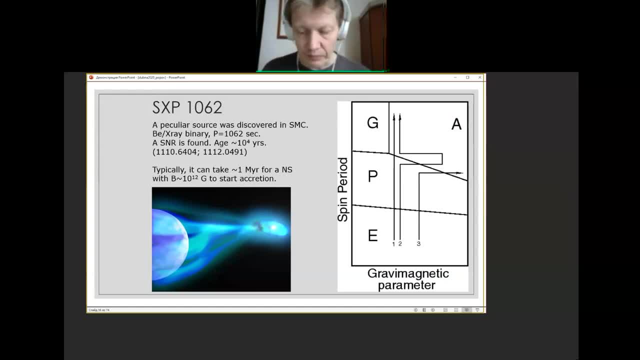 but as a cracking sources and binaries. And again magnetic field is in the game, because in binary systems we see X-ray sources, because matter is transferred from normal star to a compact object And of course this matter is plasma. So again, 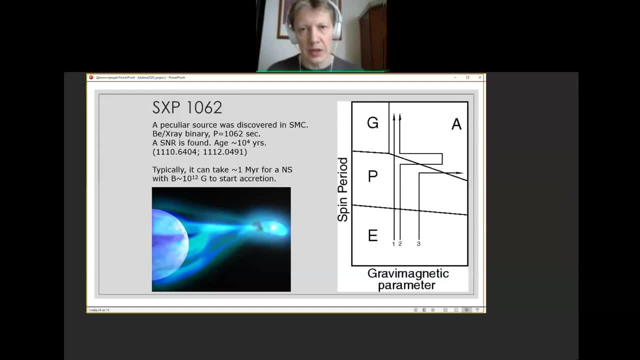 we have gas made of charged particles and they fill the magnetic field. Magnetic field is strong. So close to a neutron star, magnetic field starts to channel the accretion flow And studying properties of accretion sources we can determine the magnetic field. This is quite interesting, especially if you know the age of the neutron star you are studying. This is not trivial. Typically we see accretion neutron stars in relatively old systems. Relatively old means million years, And that's a lot. 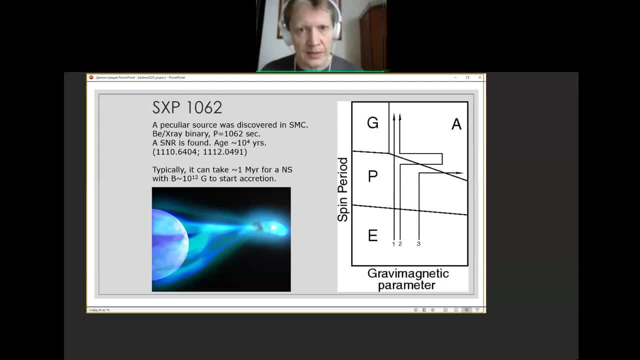 And it's difficult to obtain a precise age estimate. But in the last years, in the last 10 years, people started to find more and more X-ray binaries inside supernova remnants. Supernova remnant is the remnant of supernova explosion. 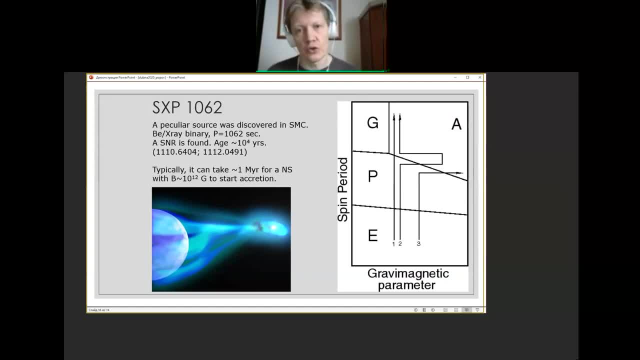 of course, And they are visible for quite a short period of time, less than few tens of thousand years. And, what is more important, if you observe, if you see a supernova remnant, you can determine its age with relatively good precision. 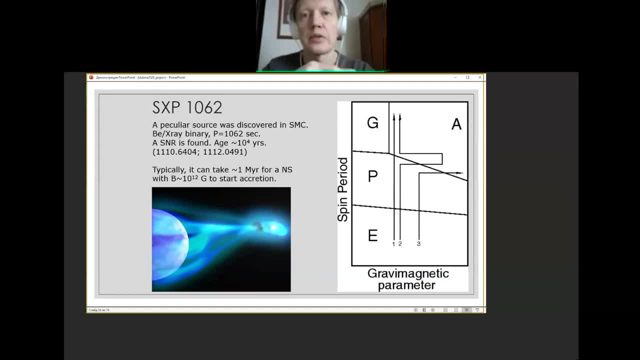 So at least with precision much better than other methods of determining a neutron star age. So nine years ago, a system was discovered in small Magellanic cloud with a very simple name: SXP 1062.. SXP means S means that it is in small X-ray. 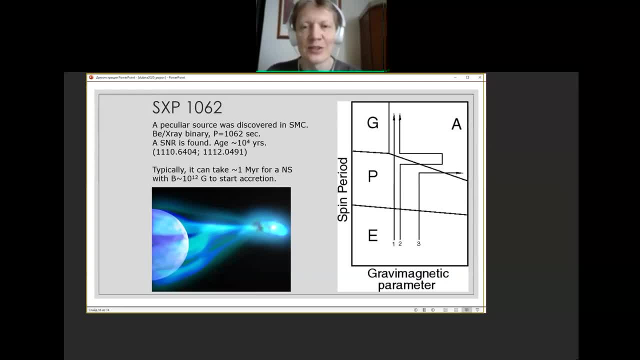 small Magellanic cloud. X means that it's an X-ray source, P that it is pulsating, And 1062 is simply the spin period and the moment of discovery, And it is in a supernova remnant, so its age is about 10 to 4 years. 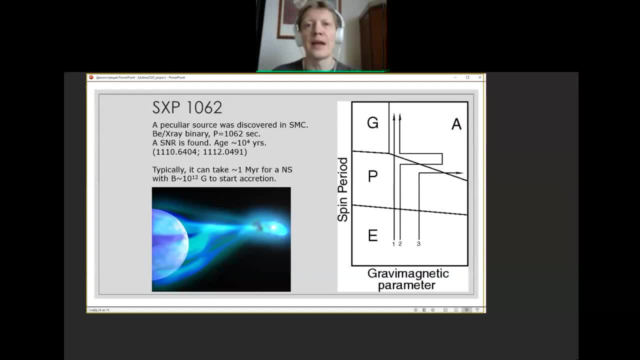 This is strange because neutron stars might not accrete at these young ages And it was necessary to find the model. how it is possible? The first guess by the authors of the discovery was that a neutron star was born with a long spin period. Long means one, two, three seconds. 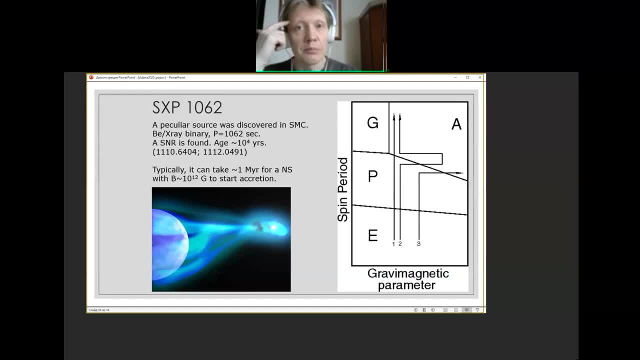 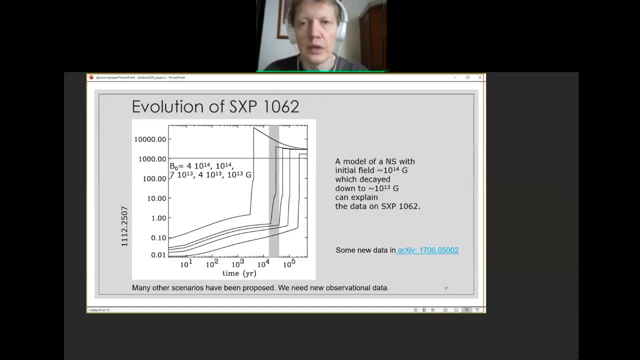 So not actually very long, but long in comparison with typical spin periods, which is less than 0.1 seconds. We tried another model. We tried to say that the neutron star was born with a very large magnetic field, So with large magnetic field. you remember the P-P dot diagram. Large magnetic field means large dot. So a neutron star rapidly spins down. But the magnetic field also can rapidly decay. So at the age of several tens of thousand years you can have a neutron star spinning relatively slowly. Not, of course, at 1,000 seconds, but at, say, a few seconds, Spinning slowly and with magnetic field decay by, say, an order of magnitude. Since this happened, since this happens, the accretion can be star. 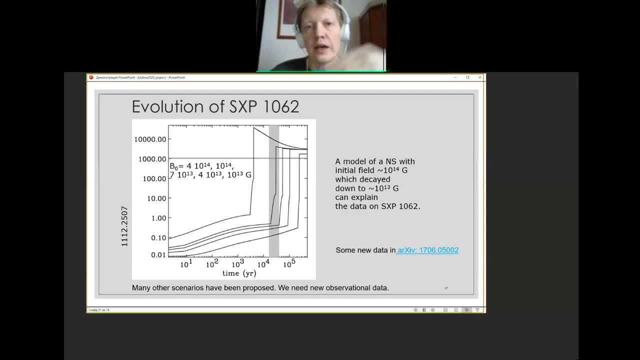 Because now the neutron star rotates slowly and the centrifugal barrier is not effective anymore. So we tried to feed parameters and indeed we found the solution. Then, with colleagues mainly from Germany, we obtained new observational data about this source, made some additional modeling and confirmed this result. 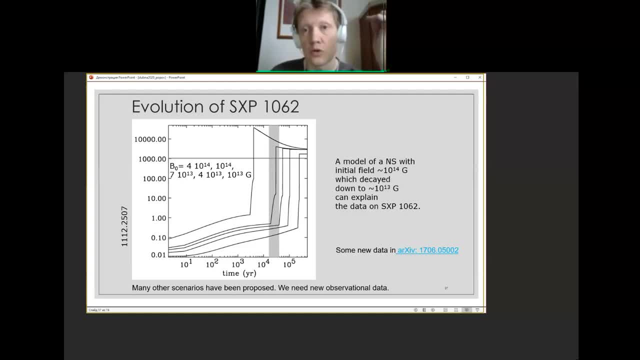 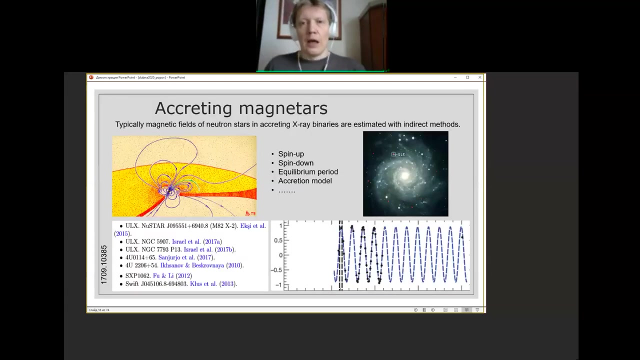 that indeed the present-day magnetic field might not be strong in this source, And rapid appearance of a neutron star at this stage of accretion can be explained by rapid magnet rotational evolution in its youth. And now it's over, because the magnetic field decay. 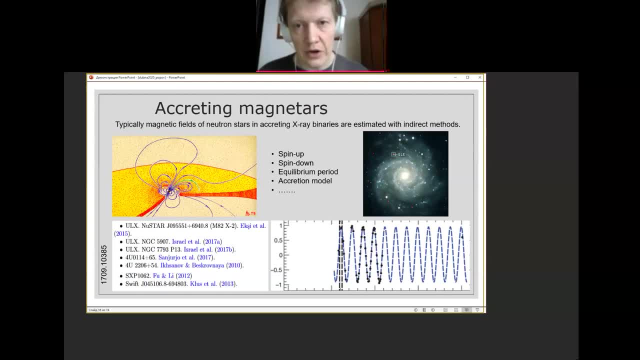 Still, there are some systems in which people suspect that an accretion neutron star can have large magnetic field. This is puzzling because magnetars and other types of sources tells us that magnetic field might decay rapidly And, as I told you, in X-ray binaries. 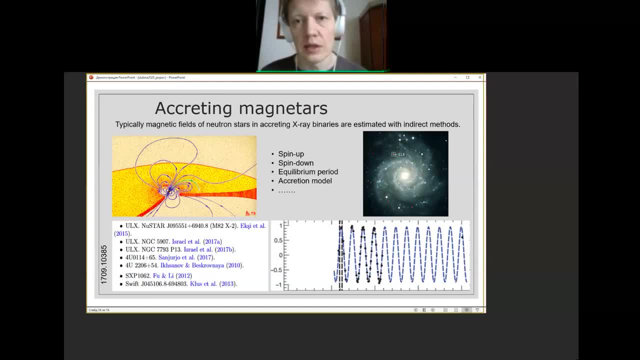 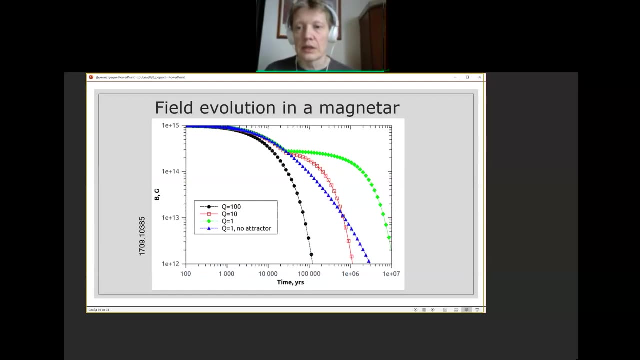 we mainly absorb sources with ages at least larger than one million years, maybe even a few million years, 10 million years. So it's very strange how you can save the magnetic field. for quite a long time We tried to play with parameters and we found out that 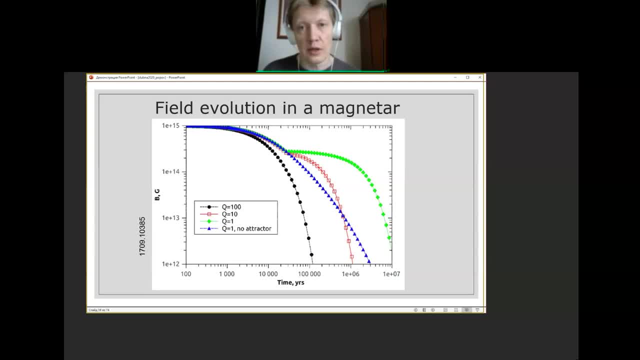 the only way is to make two assumptions. Both are necessary. The first one is that the whole attractor is working. The whole attractor is rich, So the rapid magnetic field evolution due to whole cascade is stopped in some neutron stars. And then the second assumption. is that the crust is very pure, in the sense that the level of impurities is small, and so resistivity due to impurities is not very large, So the conductivity is large. So with these assumptions we can find solutions which fit some candidates to accretion magnetars. 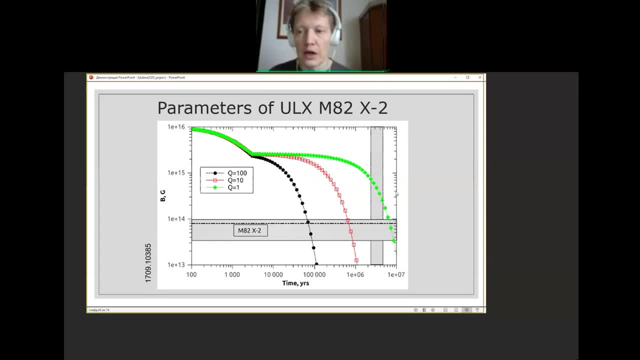 So we can save field above 10 to 14 Gauss for more than one million years. So the horizontal axis is the time scale. But this needs some not just fitting but needs some parameters which are not safe from the most popular set. 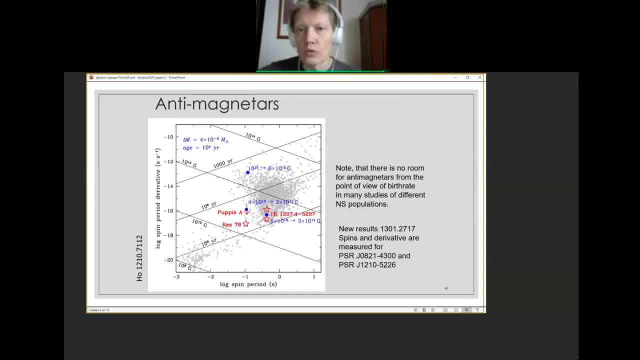 Okay, I promised to say a few words about emerging magnetic fields And let me start. So the idea of emerging magnetic fields: here I just give a general picture. even we'll not speak about our results because we don't have time. So if you look at PPdiagram, 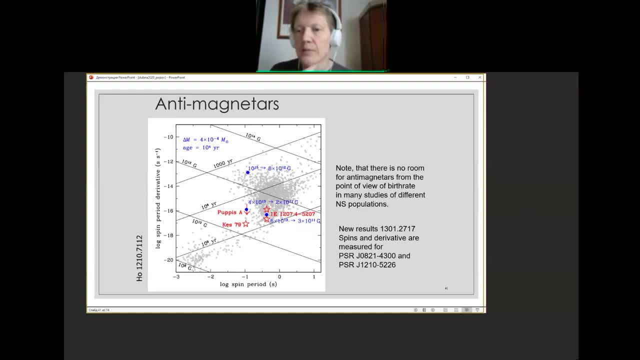 then we have sources called anti-magnets. They are found by supernova remnants, So they are called CCOs, Central Compact Objects in Supernova Remnants. Here you see three examples: PUPESA, Cas79, and this long number. 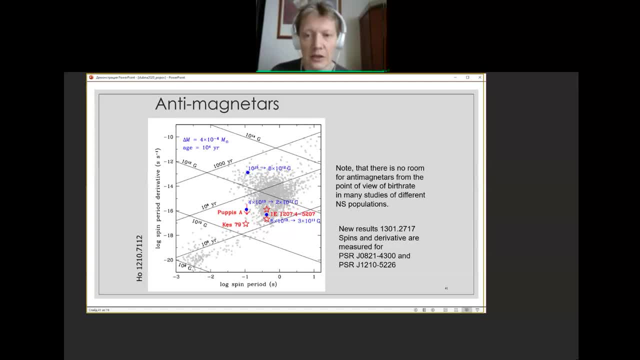 They are called anti-magneters because they are situated on the other side of this radio pulsar crowd, in comparison with magnets which, as you remember, are situated here on the top right. These sources are puzzling in some sense because they are not numerous. 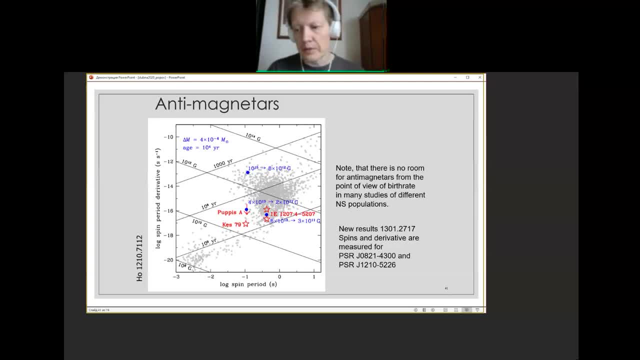 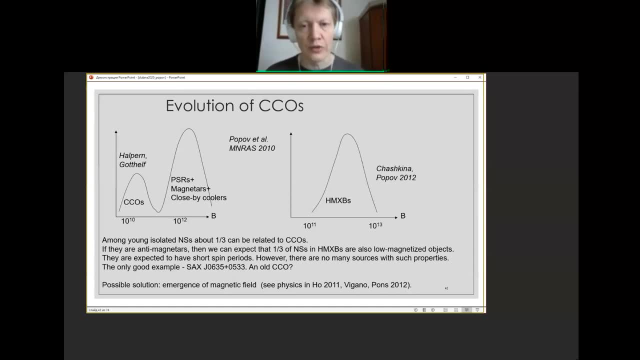 but they are very young. So if you calculate their birth rate, their birth rate is high. So if you make, say, normal population synthesis of young neutron stars, you see that magnetic field has surprising bimodal structure. So there is the main peak. 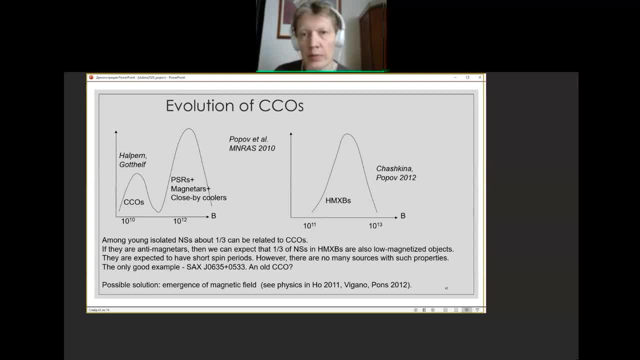 just to give you an idea. However, we can take neutron stars in X-ray binaries, in particular in high-mass X-ray binaries, And we can use different models of attrition of interaction of matter and magnetic field to derive the magnetic field distribution. 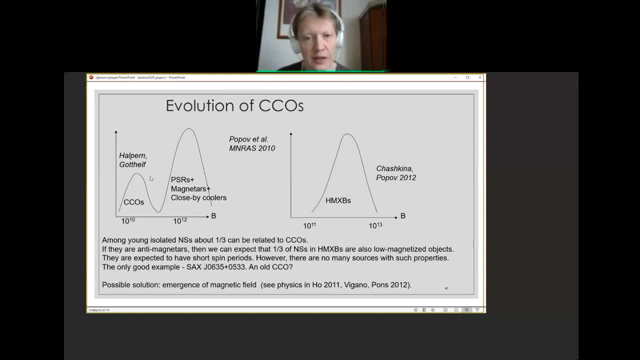 for them. And surprisingly we don't see the second peak, And it's very difficult to imagine to invent any selection effects or something else which can explain why the distribution is bimodal here and single mode here. The only idea can be that 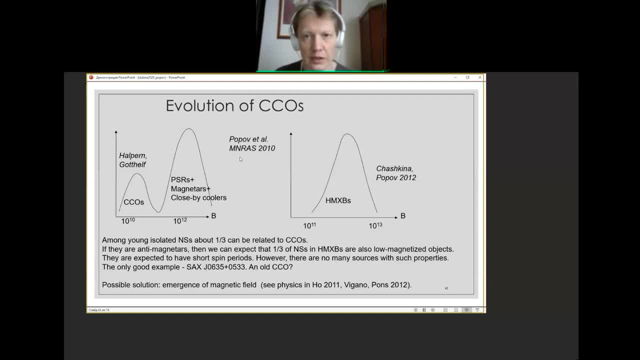 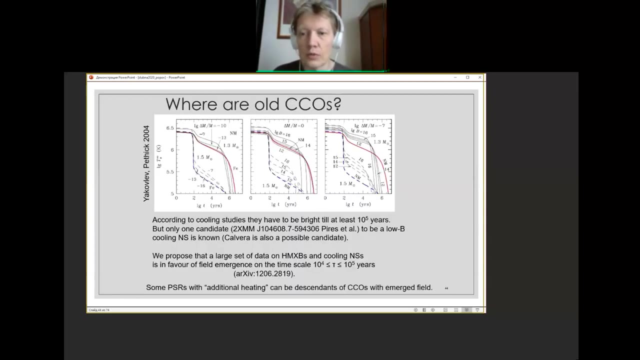 these objects are, on average, young, so less than one million years. And these objects are at least an order of magnitude older, So maybe something happens in between. So this peak disappears, but how and why? So the idea was that the magnetic field 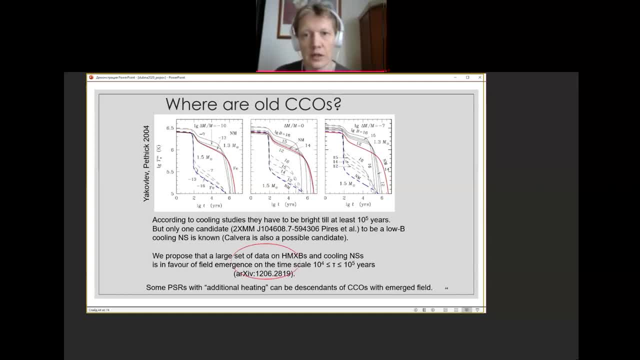 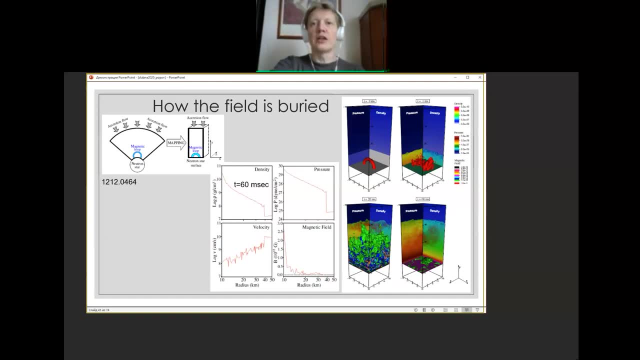 the external magnetic field of these sources is increased. Okay, let me explain why and how It is increased. because initially it was hidden. It was hidden by the process of fallback After a supernova explosion. you have a compact object form and you have a matter ejection. 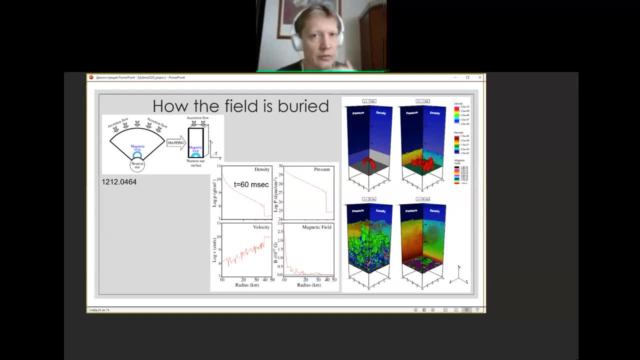 But part of this matter- maybe a significant part of this matter- will not go to infinity. It will fall down because of gravity And this process started to be modelled in this decade And in early models it was quite simple. You have a loop of magnetic field. 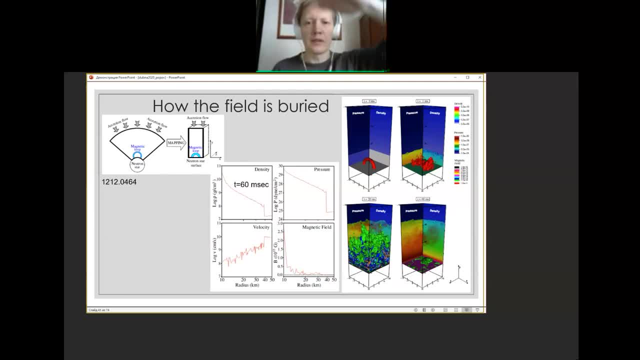 and so it's 1D and you have a kind of wall of matter falling down And it happens very quickly. So I don't know, maybe you don't see the timescale, So zero millisecond, one millisecond, 20 milliseconds. 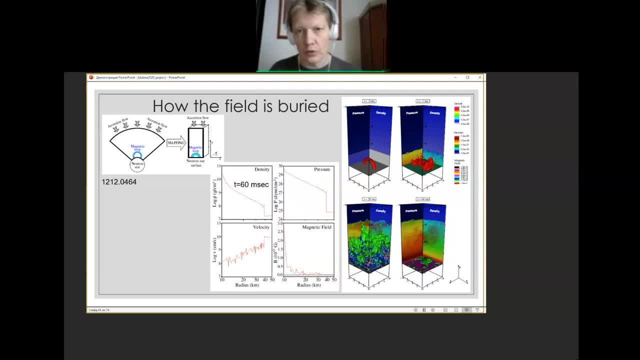 60 milliseconds, So everything is finished in a few tens of milliseconds You have this matter falling down. It's a huge flow of matter- Well huge in comparison with the magnetic field energy- And it covers and screens the magnetic field Because it's plasma. 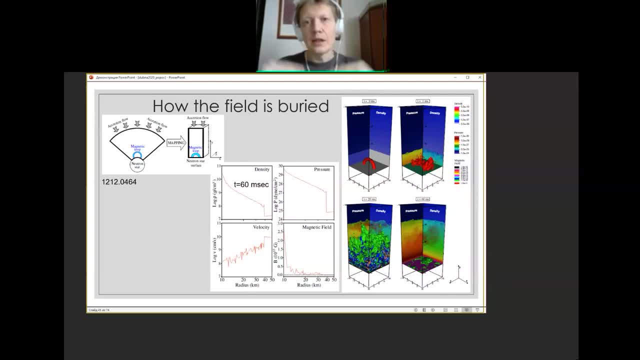 It's conducting material And then slowly, magnetic field, which is now confined in the crust, starts to diffuse out through this envelope, which is not actually that thick. Well, it can be thicker or thinner, but generally magnetic field can diffuse out. 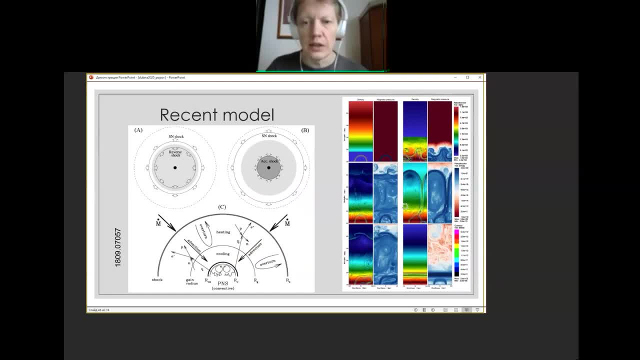 Recently it was studied in more details. Now not in simple 1D models, Just to show you beautiful pictures. So just want to illustrate that the model becomes more and more detailed, But the general conclusions are the same. So the field is diffusing out. 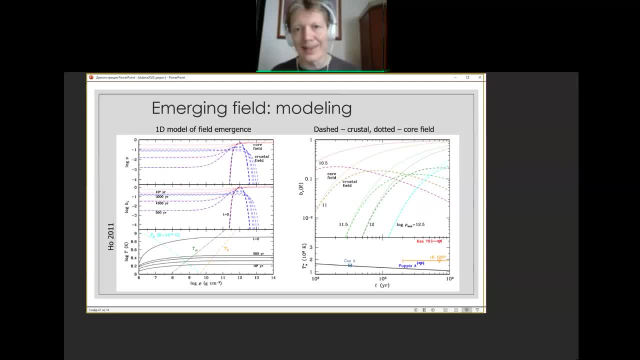 And for an external observer it looks like increase of the bipolar magnetic field. What is the timescale of this diffusion? Of course it depends on how deep in the crust you put the magnetic field. What's the thickness of the outer layer? 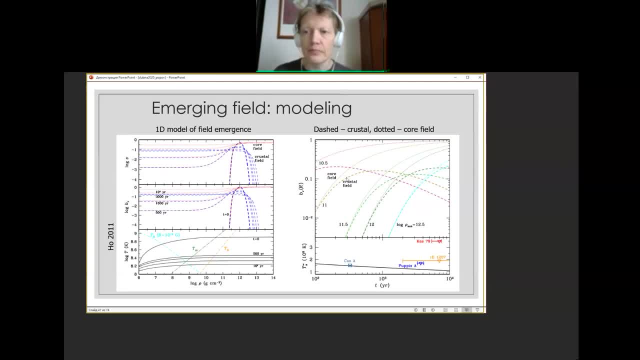 If the layer is relatively thin, then the field diffuses out on the timescale of 1000 years, But if you take more realistic levels, then the time of diffusion is larger. This was the first simple model, However. I recommend this paper. 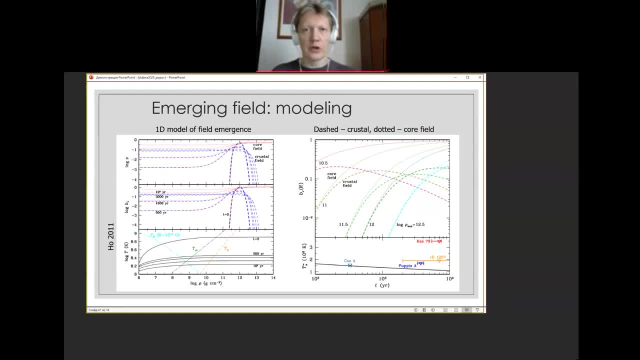 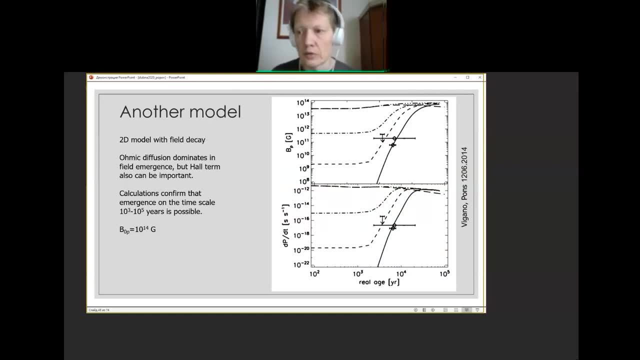 by Vinh Ho, because it's a very clear, let's say, explanation of physics. However, if you look on more realistic models, for example by the Canoan Ponds, then the time it takes to the field to diffuse out. 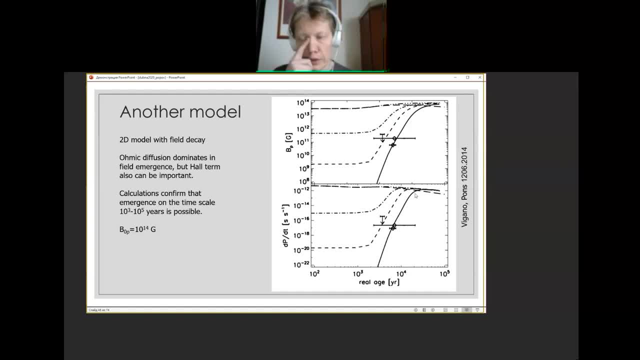 is larger And it's more than 10 to 40 years, And what we see here, these three objects here, are anti-magneters. So actually they're not maybe anti-magneters, So they're not objects with the low field in the crust. The field in the crust is just hidden And then it slowly diffuses out and we observe sources at this stage when the field is still hidden by this outer envelope. But later on they will appear as normal radio pulsars or even as magnetars maybe. 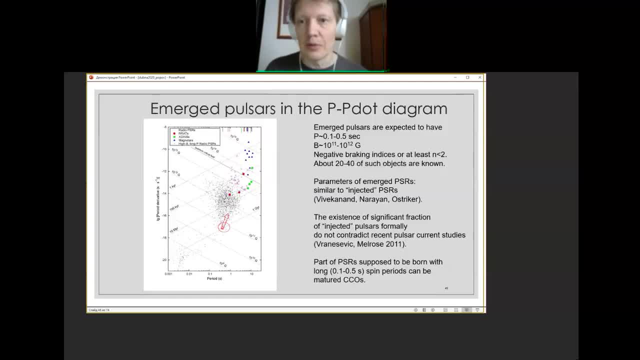 And we have one interesting example maybe for this source. But at first I just want to show that if we're looking for such objects, then they have to move up in the PP-dot diagram And maybe we have examples. There are two radio pulsars. 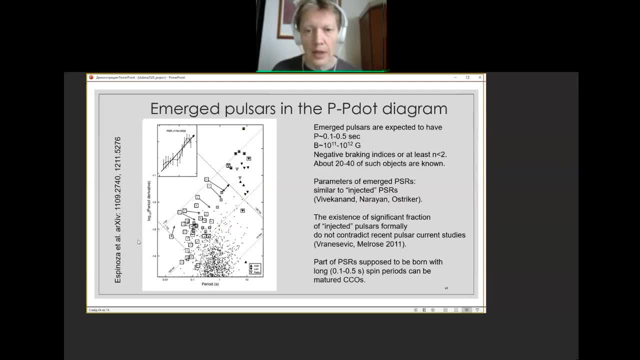 which seem to move up. It is observed because the second derivative is known And it shows that the first derivative is growing, which is not normal for a radio pulsar. The only explanation- well, not the only, but the main explanation- is that the external dipolar field 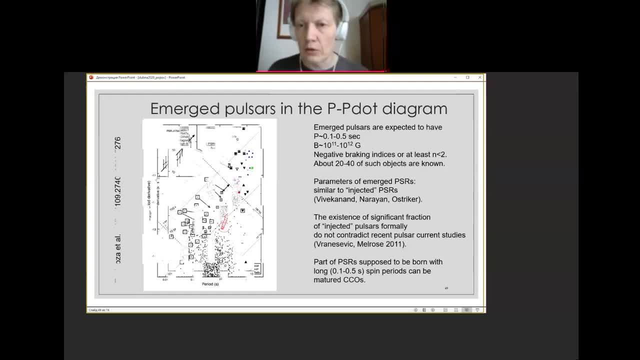 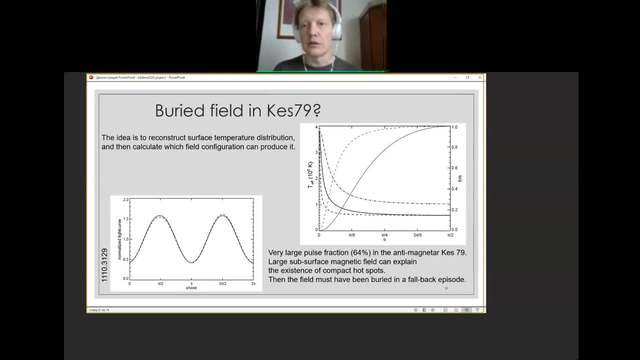 is increasing and it can happen because of this moving up. Okay, I'll skip this. There are some indications that in this antimagneter, the magnetic field is strong in the crust because it shows very strong pulsations in X-rays, which is due to heating. 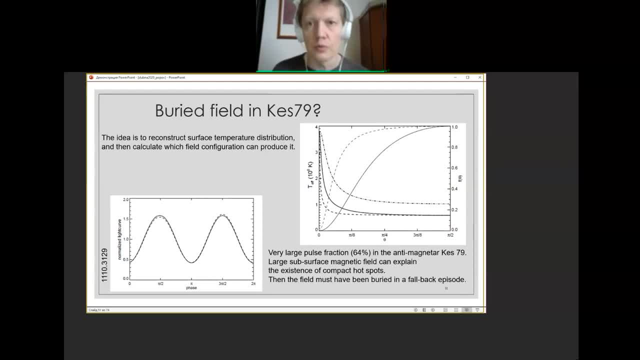 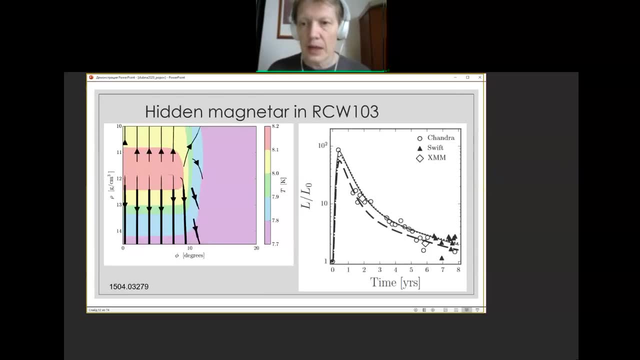 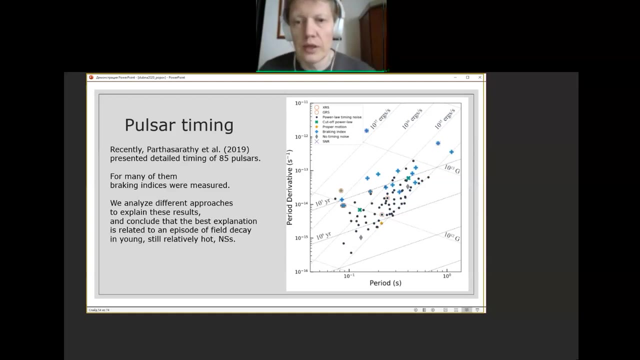 of the crust. It is supposed to be due to heating of the crust by strong, decaying magnetic field in the crust. I'll skip our results on RCW-100-03 and come to our recent results. We just well, the paper is not out. 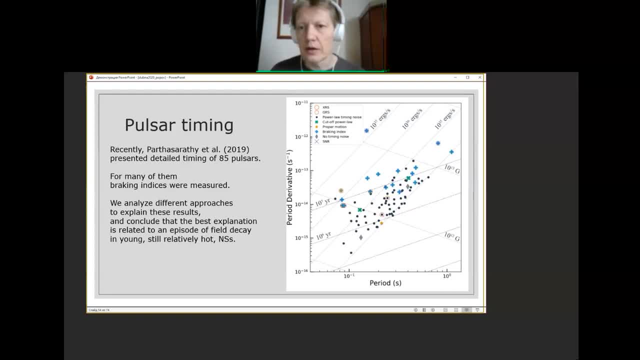 It will be published in December, but in the archive it appeared less than two months ago And the second paper is coming this week. Okay, So people continuously monitor radio pulsars to obtain more and more data and to make it more and more precise. 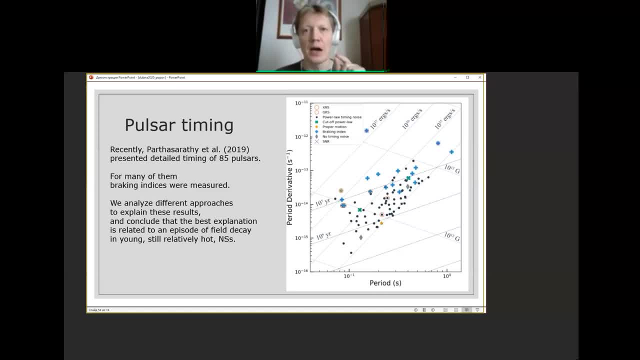 So, in particular, people are interested in how pulsars are moving in typical time. So some are moving towards right and down. This is normal direction, But some are moving up. Anyway, they are moving right, That's inevitable. They are slowing down. 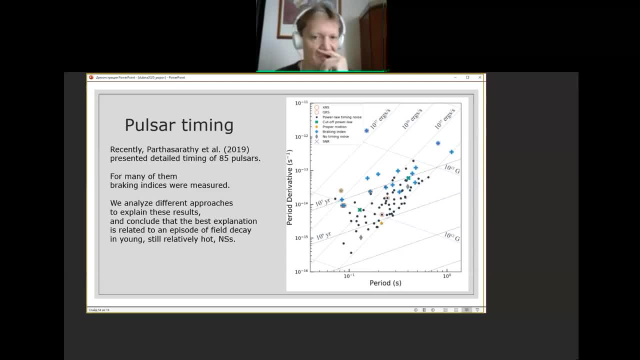 But up or down it depends. And this year appeared some new set of observational data So people made these observations for quite a long time. Last year they presented this set of radio pulsars. They are shown on this PP-dot diagram. 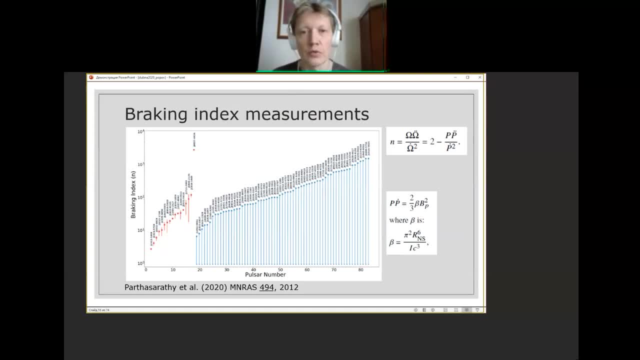 And this year they presented measurements of so-called breaking index. Breaking index is just a combination of the spin frequency- second derivative- and first derivative, And of course, you can rewrite it in terms of period- first derivative and second derivative. 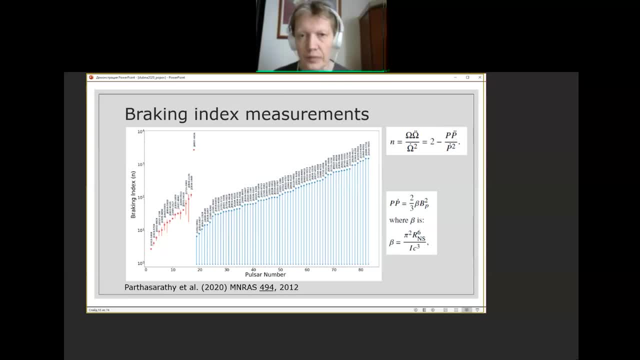 Normal value is 3.. So this is the classical value from magneto-dipole formula. However, they found out that for all- well, for the main part, for most, I would say for most- of radio pulsars for which they obtain measurements, 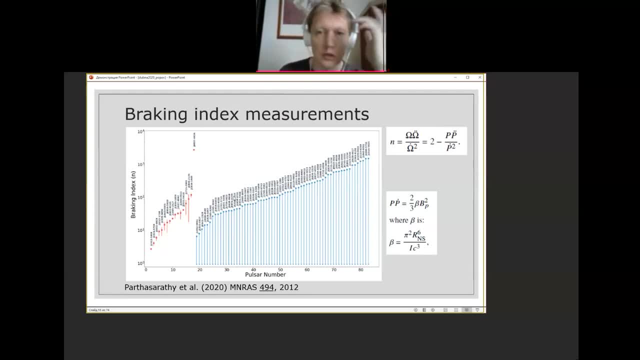 not upper limits in blue upper limits as shown. I will not discuss them, But for those for which they obtain measurements, breaking indices are large, significantly larger than 3, larger by another of many. It's interesting to find explanation for it. 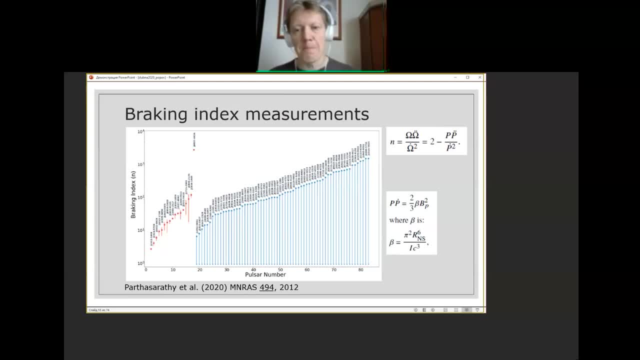 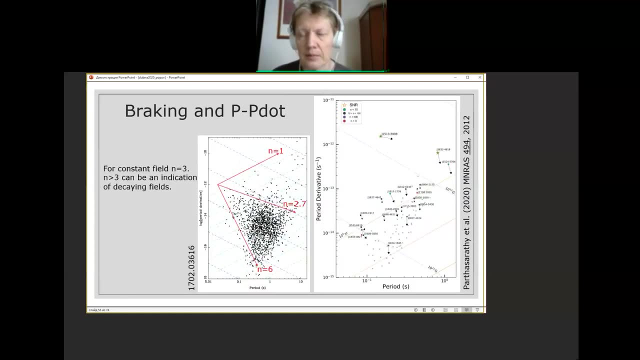 And it's important to notice that mostly these pulsars with large breaking indices are young. So we made additional modeling to show the same thing. Here I just illustrate how pulsars with different breaking indices move And, of course, if you have breaking index. 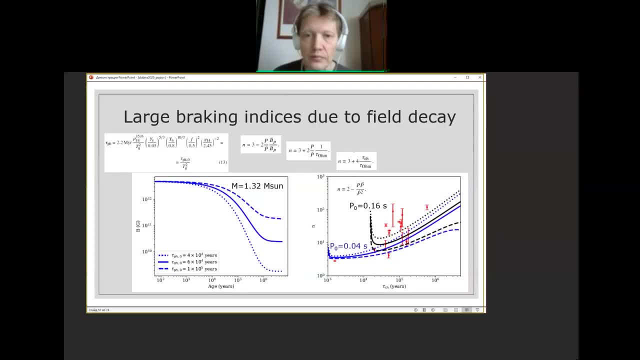 say 100, the pulsar is nearly moving down. We tried to model breaking indices in our slightly advanced model of magnetic field decay, which goes together with thermal evolution and all the rest, And we found out that we can explain these large breaking indices. 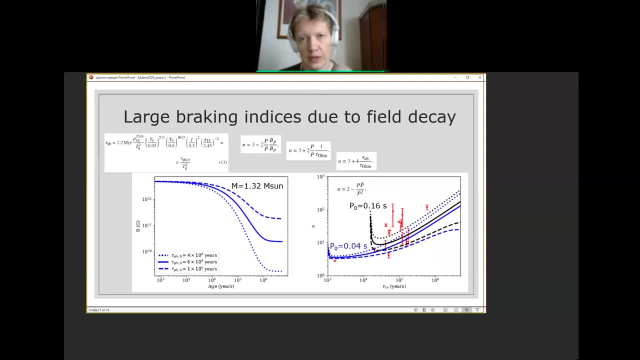 if we observe these pulsars at a short episode of magnetic field decay in their youth. So on the left plot you see how magnetic field is evolving And on the right we see how corresponding breaking indices look like versus characteristic age. So maybe I'll show. 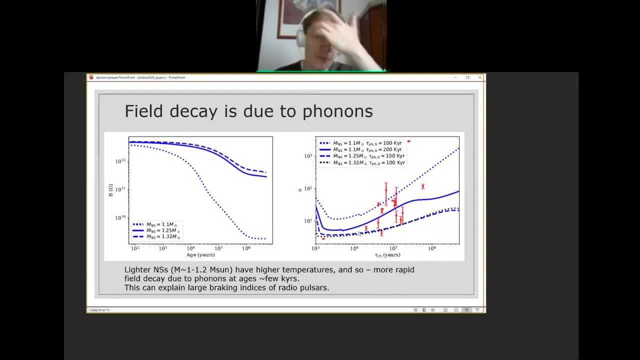 you this picture. So again, field evolution on the left and magnetic field and breaking index versus the characteristic age on the right, for different set of parameters, for different masses, And we can find the solution even for well large, even for breaking indices. 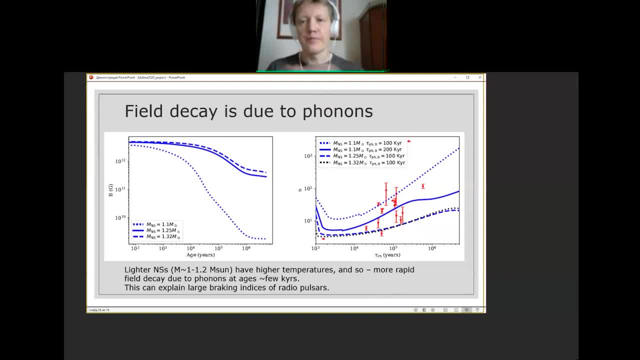 close to 100, if these neutron stars have relatively low masses. low mass neutron stars cool down slowly, So decay due to phonons is important for much longer time, And so we can observe we can find significant number of such neutron stars. 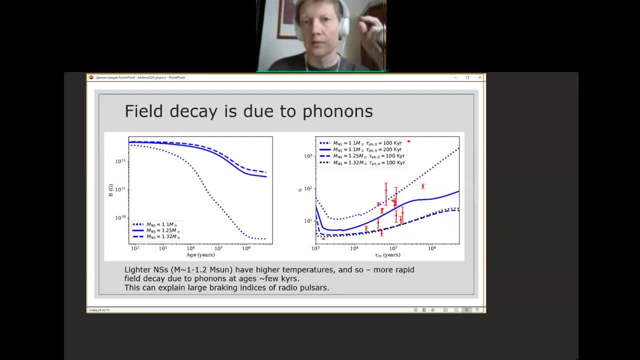 at the stage of magnetic field decay and an episode of magnetic field decay just by a factor of two, So we don't need more. Well, maybe three. It goes together with: well, it is described by large breaking indices. That's better phrasing. 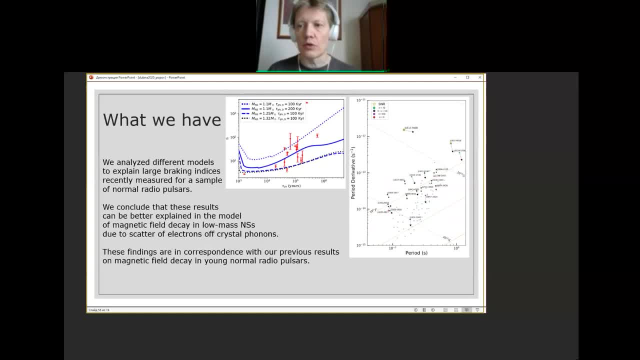 Okay, So I think my time is out, So I just summarized that in our recent paper we, in our opinion, found new confirmations in favor of new confirmations to an episode of magnetic field decay in young hot neutron stars. 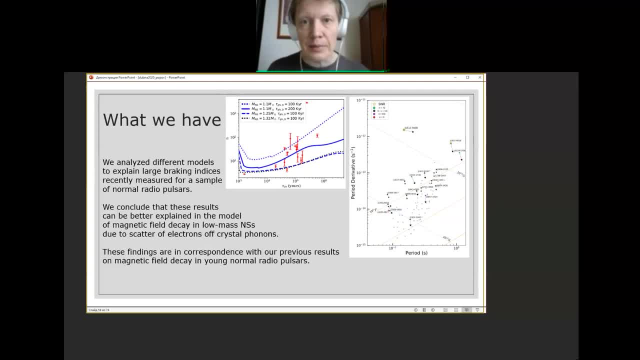 due to scattering of phonons. This episode is over in several hundred thousand years because neutron stars cool down. even low mass neutron stars finally cool down And it looks like. even in normal radio pulsars we see evidence for magnetic field decay. And finally, 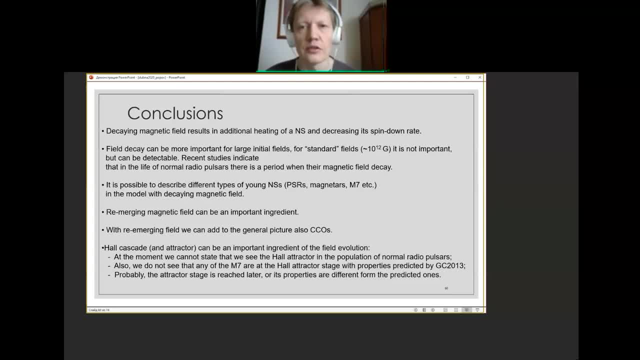 it helps. I will not read my conclusions, I will leave it here. Finally, we can explain more and more populations, subpopulations of isolated neutron stars in the framework of evolving magnetic field going hand by hand with thermal evolution, with realistic mass distributions. 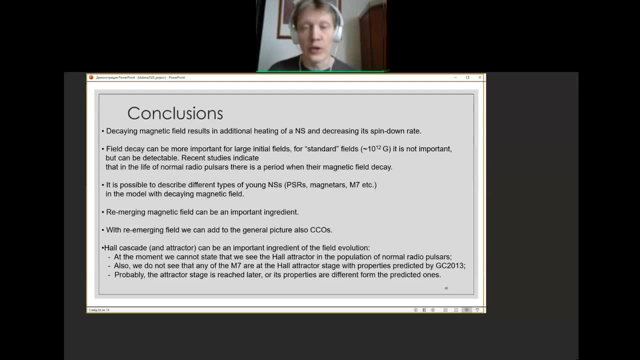 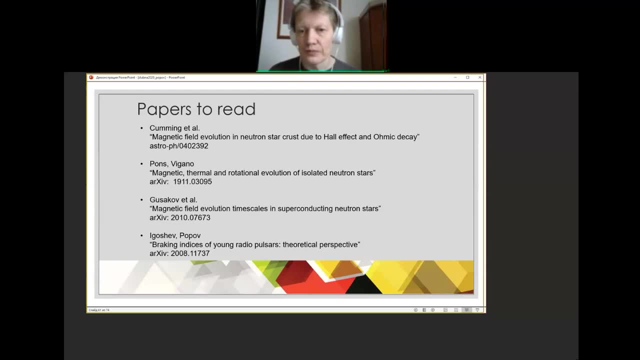 and so on and so on, coming finally to realistic equations of state, which is interesting, to nuclear physics and particle physics. Just to guide you in the sea of interesting papers of magnetic field evolution, I want to mention mainly two: The paper I mentioned earlier. 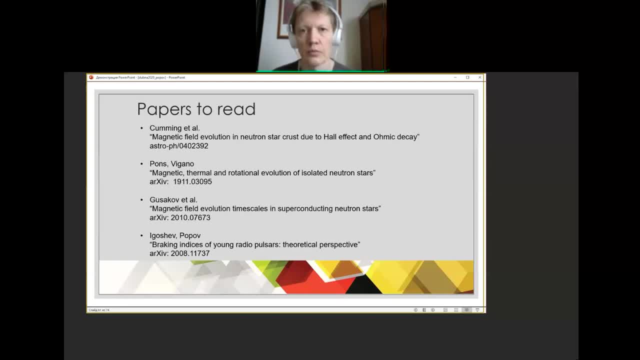 with the detailed description of physical processes, with detailed and clear description of processes of magnetic field decay in the crust, Then a very recent review by Pons and Viganò about magnetic thermal and rotational evolution. so we put those all together. Then I want to remind you, 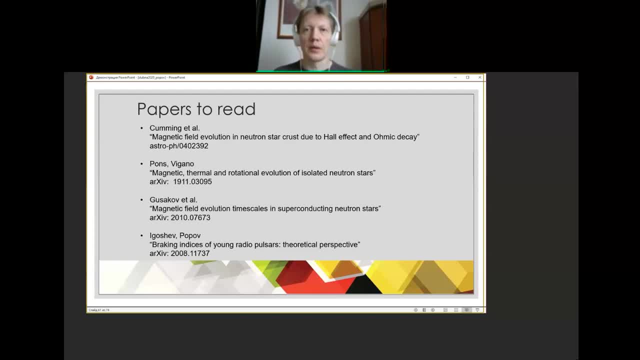 about a very interesting recent paper by people from Iofi Institute about field evolution in the core, which I think is the future of neutron star studies in this respect. And finally, I refer to our recent paper in which we found, as we think: 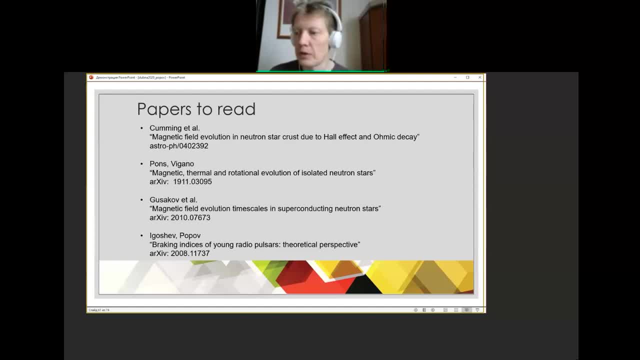 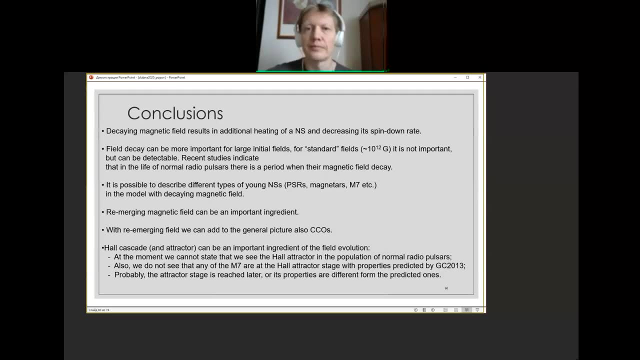 new evidence for magnetic field decay in radio pulsars. Okay, thank you, I'll stop here and put my conclusions on this paper. If you have questions, I'll be happy to answer. Thank you very much. Thank you very much, Yeah, please, participants. 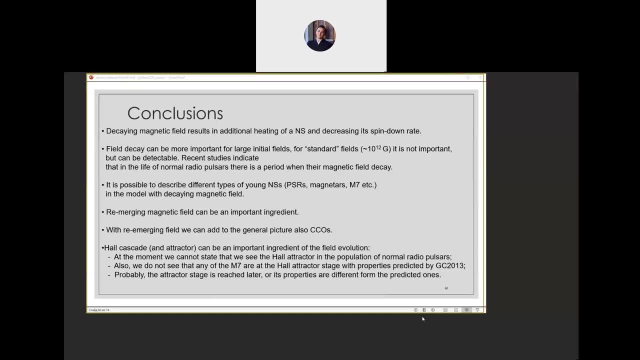 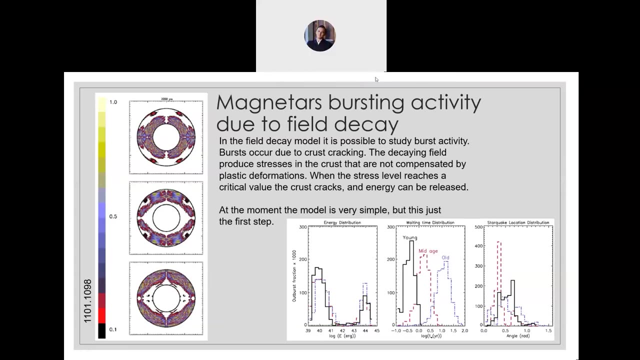 now. we are ready to listen to your questions. If you have questions, please raise your hand and we will give you. Okay, We have one question from the chat from Ilnur. He asks the following things: Can the accretion of matter? 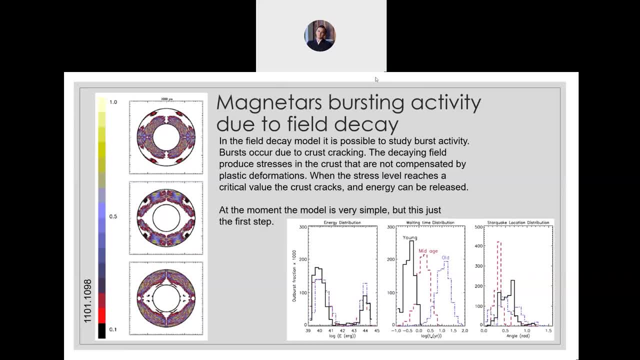 and the consecutive bursts somehow give additional energy to increase the magnetic field? I would say hardly. Even opposite. attrition and the heating of the crust due to attrition can enhance magnetic field decay And, in many models of long-term magnetic field, evolution, which finally leads 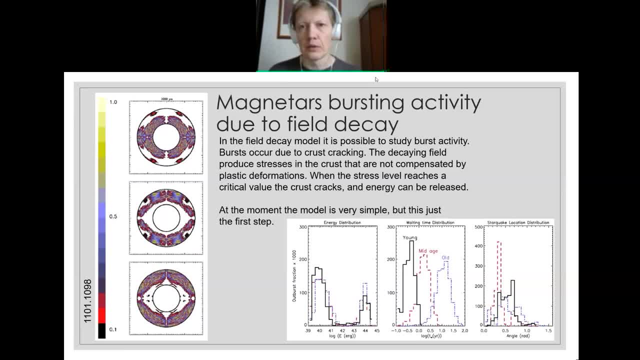 to millisecond radio pulsars. people suppose that heating of the crust by attrition and binaries finally results in magnetic field decay. To increase magnetic field you need- well, you need- 3D movements, You need some kind of dynamo mechanism. 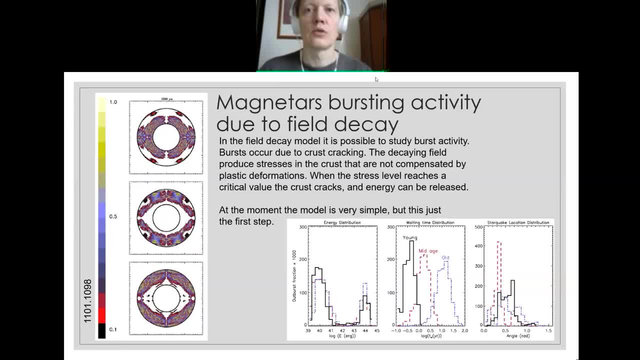 And the crust is solid. So if you make the crust liquid somehow and then put on convection and everything and enhance magnetic field in the crust, then it would work. But normal attrition episode cannot do it with a neutron star crust. So I would say that 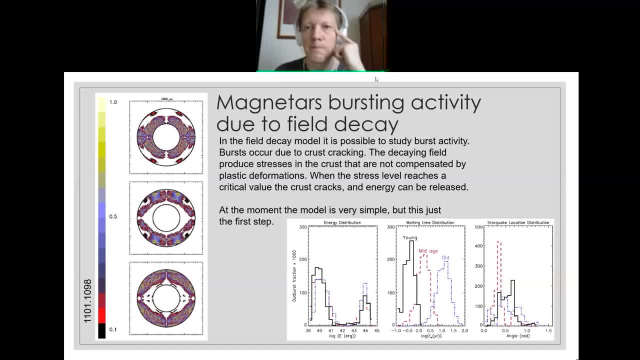 accretion cannot enhance the field. Okay, Any questions? Okay, let me Well, yeah, I have some kind of maybe naive question. So, first of all, thank you for the lecture And at the very beginning, maybe on the slide number two: 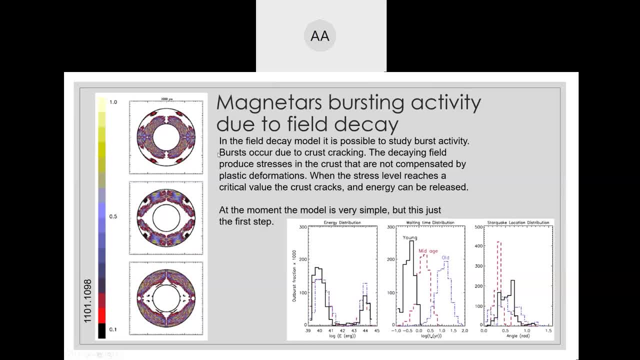 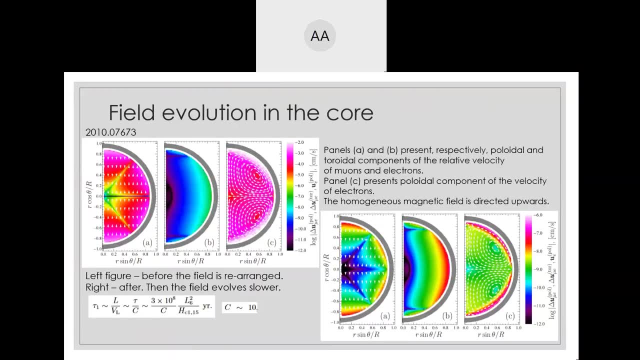 you showed us these nice pictures of different velocities inside the core And I would: Yeah, yeah, these pictures. So I was just trying to understand, like, is it So this pictures ABC, is it like a time evolution of the core, or is it different structures? 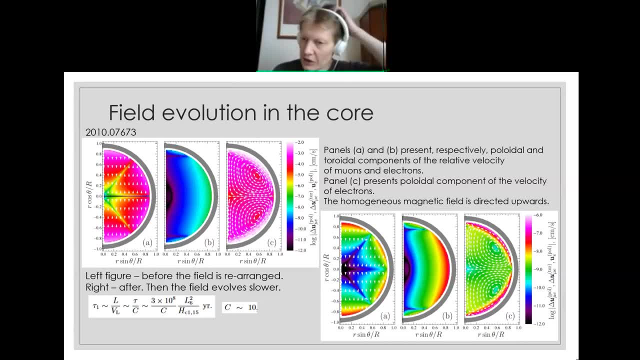 Yeah, yeah, Sorry, I didn't. Indeed, I didn't describe it. It is briefly described in the text on the slide. So two pictures, on the left and on the right. they correspond to two different models, So the left to the earlier period. 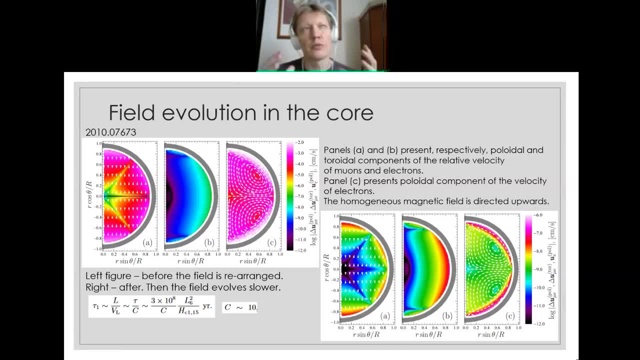 to the period before thermal relaxation state, not thermal relaxation of the core in the very beginning. but it corresponds to say young, hot neutron star with an age maybe a few hundred years And the right picture corresponds to an older neutron star with an age typical. 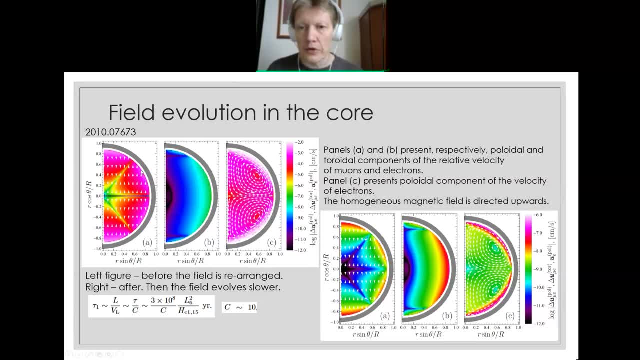 to your radio pulsar And three panels on each picture corresponds So panel A to relative velocity of moons and electrons, And on panel A it's poloidal velocity, On the B toroidal velocity, relative velocity. And finally panel C shows 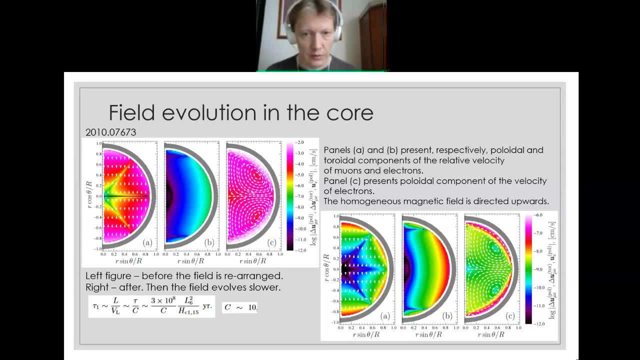 poloidal component of the electron velocity, So it's not relative, but just the velocity of electrons. So there are complicated movements of particles on top, of course, of diffusion, which also takes place there. And Yeah, So that's it. 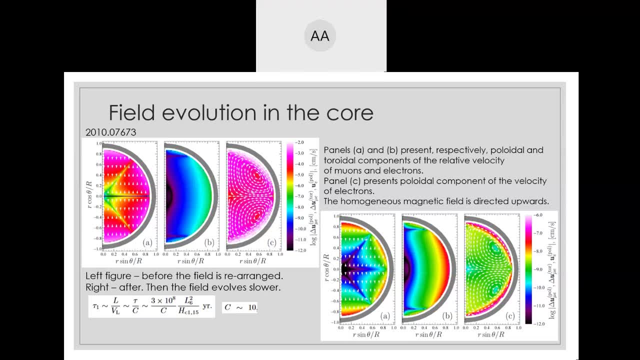 Uh-huh, Uh-huh, So maybe another question. So So these types of These types of relative velocities give me an idea, like maybe there are some kind of a stable flow inside the core or it is just some kind of random fluctuation. 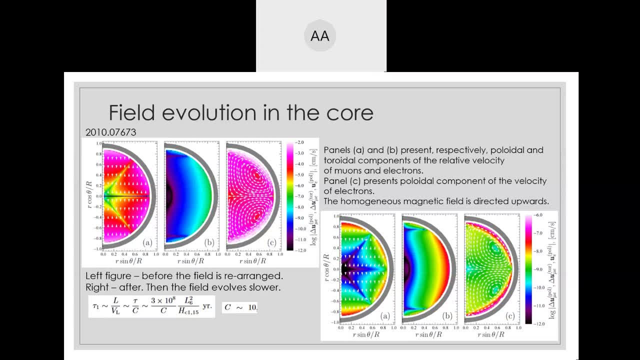 So are there any, let's say, stable flow structures inside the core? Yeah, I would say that yes, They are stable flows which are evolving, of course, And that's why there is magnetic field evolution. Yes, Especially when you look 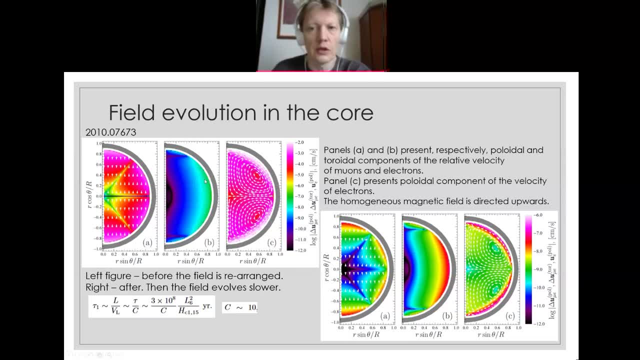 on panel C for electron poloidal velocity. it's really a stable flow, Uh-huh, Thank you. Okay, Then I have also one, I guess, stupid question. The question is: can systems such as neutron stars can be detected in our experimental installations? 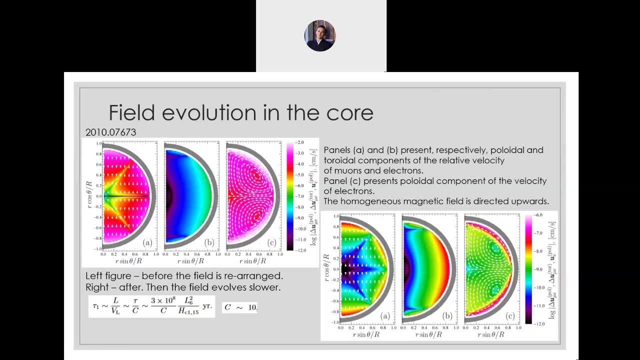 Because I heard from the nuclear physicist about the compound neutron nuclei, So could you comment? Well, I suspect that at the conference you've had better specialization of neutron stars, So I think it's possible that neutron stars can be detected in our experimental installations. 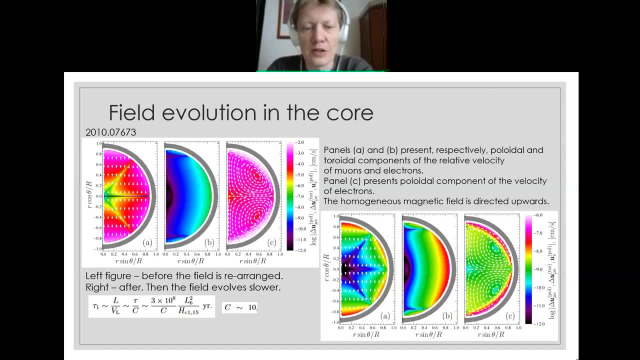 because we have better specialists to answer these questions. But of course, experiments can help to probe different aspects of equations, of the equation of states, or different equations of state, And this is one task for Nika and Fair, as far as I know. But really to make some kind of analogous of neutron star in the lab is not possible. People try to make something similar but to study really some particular aspects of neutron star evolution. For example they made the kind of neutron stars from superfluids. 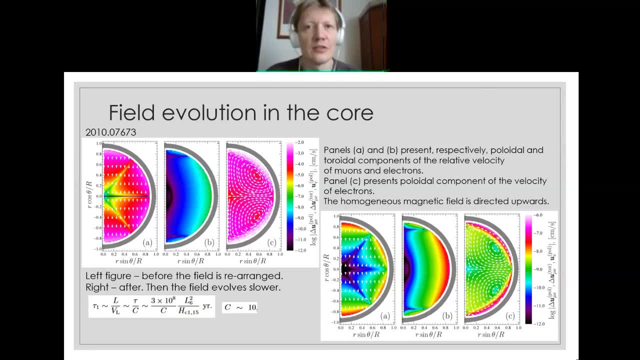 to study rotation of superfluids because it's important for neutron star, But that's quite a different subject, completely offset from, say, nuclear physics. in this sense, So I think that laboratory physics is really important for astrophysics, But typically people